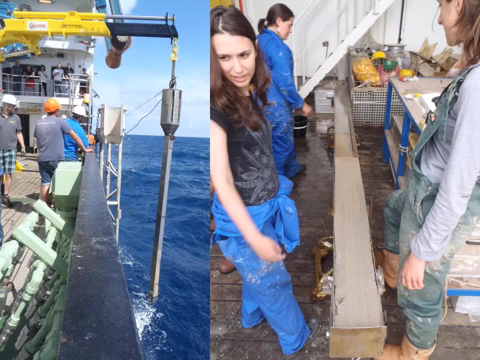 This is called a Castancora and that recovers, kind of you can see. you see, this length of mud has been recovered by these scientists here, So it's kind of this is the kind of archive that we're going to be talking about mostly today. 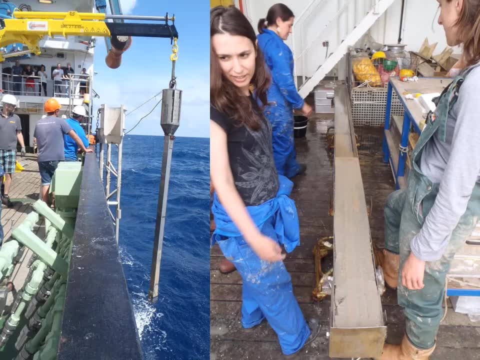 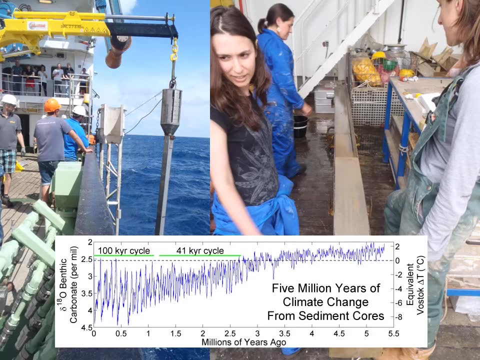 Kind of deep sea sediment cores And what kind of geochemical information we can get out of them. So usually paleo folk, kind of people that are interested in paleo climate kind of measure, some kind of wiggle down core and try and interpret that in with respect to climate. 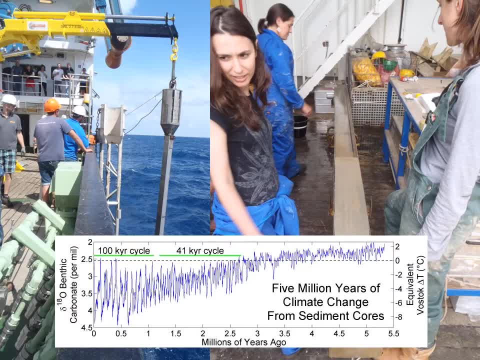 And quite often I mean you can see, this is a record, a composite record of a number of marine sediment cores using oxygen isotopes, And hopefully you'll remember back to the oxygen isotope lecture, how those work and what those might be telling us about climate. 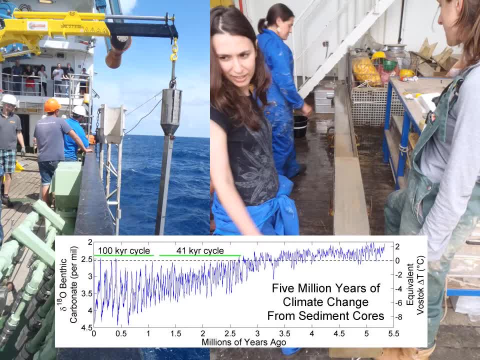 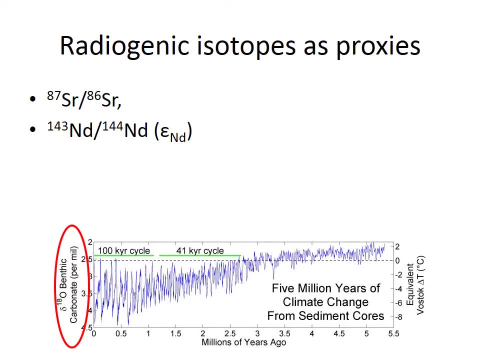 Potentially in terms of temperature Or the amount of ice on land. But today we're not going to be talking about oxygen isotopes, So we're basically going to be just using radiogenic isotopes as the vertical axis on our kind of wiggle of proxies through time. 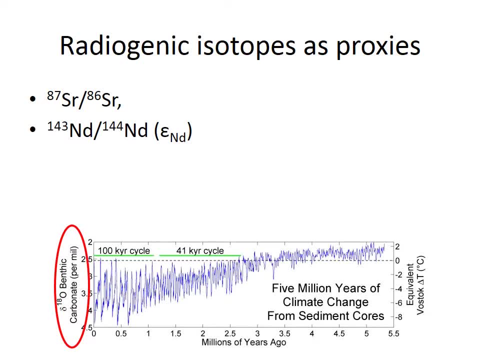 Okay, so the ones we're going to focus in on are strontium isotopes and neodymium isotopes, So you should be fairly familiar with strontium isotopes from Jeff's isotope-a-thon that he had two weeks ago. 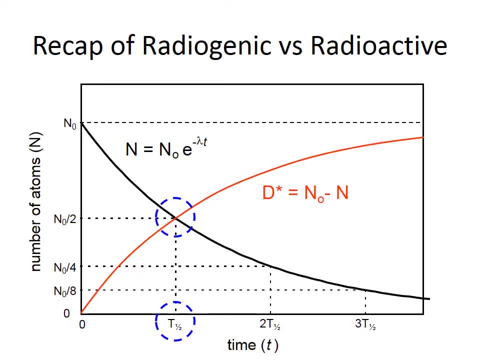 Maybe. Anyway, So just to give a quick recap of what we mean by radioactive and radiogenic isotopes. So it's basically so: radioactive is like the isotope, the parent isotope that gives off radiation and produces a daughter isotope which can be thought of as radiogenic. 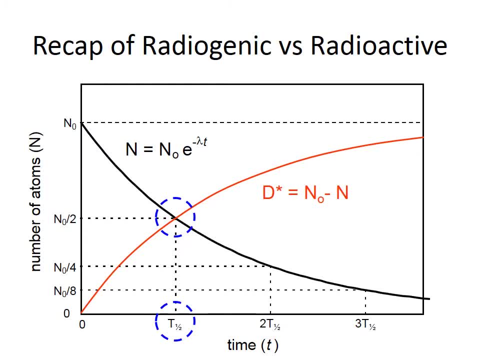 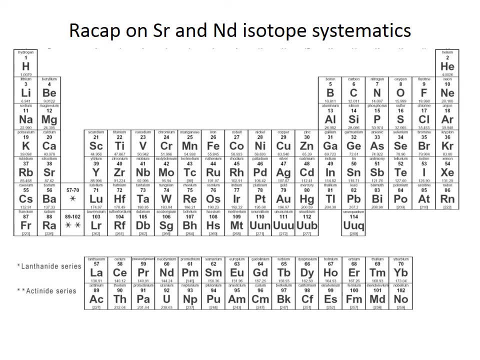 That's when it comes from radioactivity. So in this case, we're looking at making use of isotopes that make up the red curve on this diagram here. So to recap, Strontium- Oh, this has got animations on it. 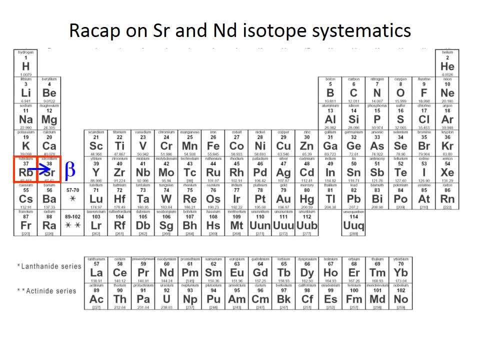 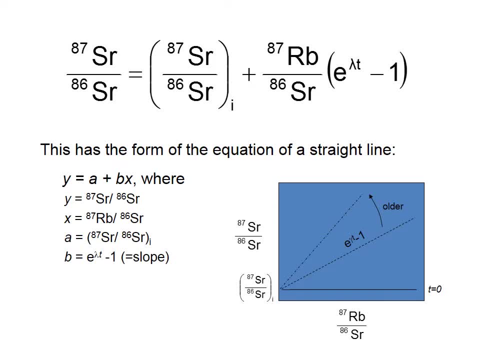 So rubidium decays to strontium with some unfeasibly long half-life And basically you have the strontium-87 comes from rubidium-87.. Okay, And then we normalize all of our measurements to a stable isotope of strontium: strontium-86.. 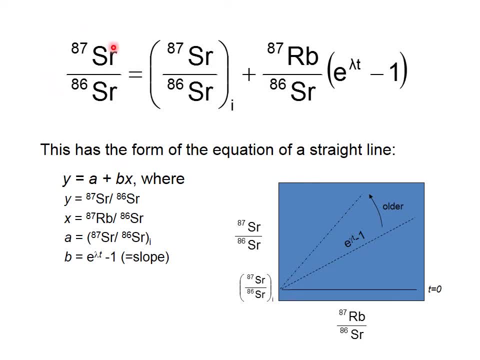 So over time, the strontium-87-86.. The strontium-86 ratio will change, so will increase through time as the rubidium decays to strontium, making this ratio bigger, Okay, And basically what we're doing is that the rate at which this number here increases, okay, depends on the rate of radioactive decay. 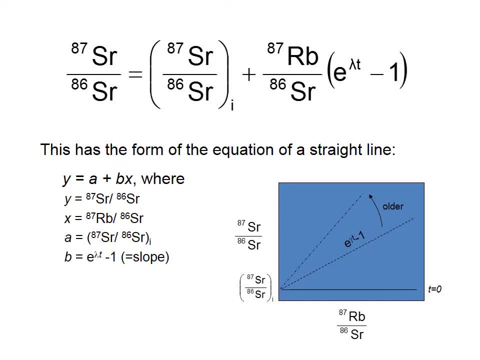 Okay, Which is fairly constant, But also the ratio of rubidium to strontium in our sample. So if we've got something with a very, very something down here with a very, very high rubidium to strontium ratio, it will increase. 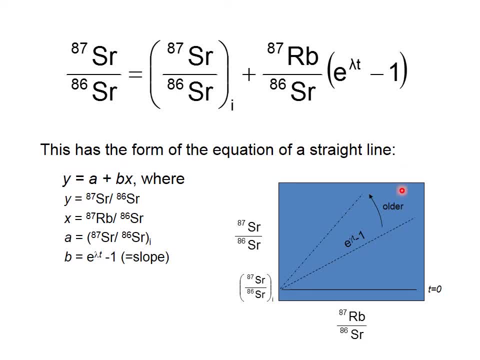 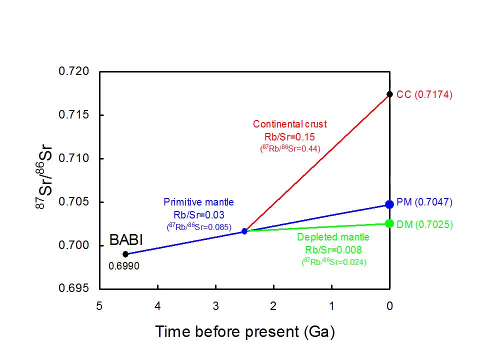 It's 87-86 strontium ratio, more quickly than something with a low rubidium to strontium ratio. Okay, And that's quite important. So if we look at how stuff has evolved through time, Okay, So basically the bulk earth has evolved along this blue line, which is basically, you know, all of the rubidium in the earth is decaying to strontium. 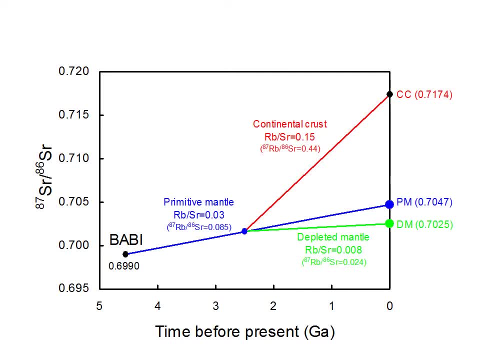 So this 87-86 ratio increases through time, But then at some point in time in this point, maybe 2.5 billion years, A couple of years ago- we have some events that maybe separates out our rubidium and strontium into different reservoirs. 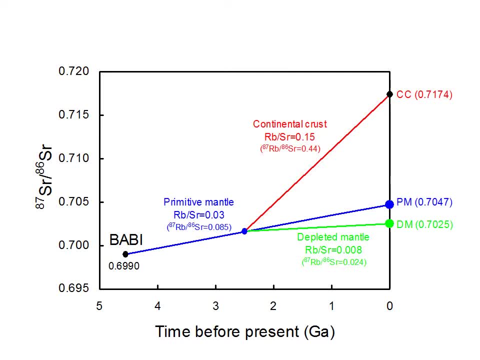 So if you form continental crust, you should know from the stuff that Jeff's been doing that rubidium is more incompatible in a melt of the mantle. Okay, So if you melt a little bit, if you melt a small amount of the mantle, okay, the resulting kind of liquid that goes on to form the continental crust. 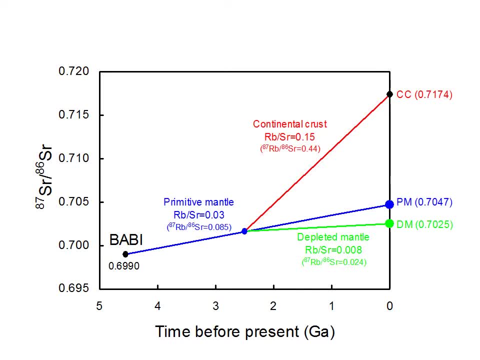 will have a higher rubidium content than what you started with. Okay, So that causes the continental crust to have a higher rubidium-strontium ratio. So over time the 87-86 ratio increases faster than the bulk earth. 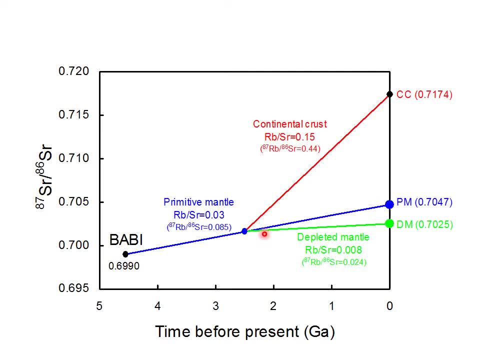 And then what's left behind after you form the continental crust is the depleted mantle, And that increases at a much slower rate because you've essentially removed most of the rubidium from the mantle. Okay, So That that does. the rubidium that's left still decays and produces 87-strontium, but at a lower overall rate. 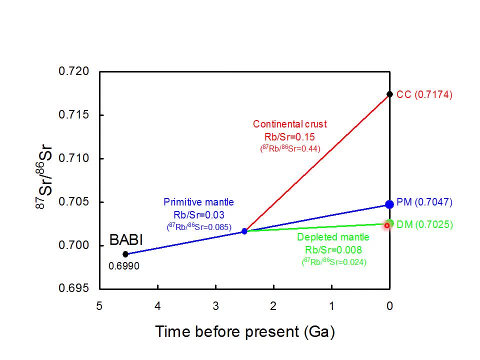 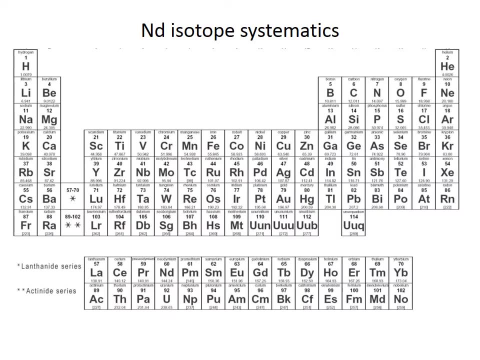 Okay, I should point out that this line is still going up. Okay, This is still increasing. You can never, on this diagram, have a line that goes down. Okay, Because you can't undo radioactive decay. Just briefly, the neodymium isotope system works in a very, very similar way. 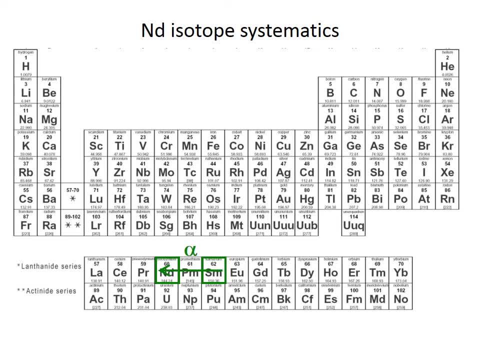 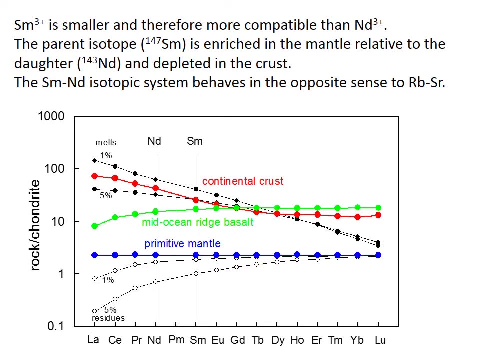 So in this case samarium-147-something. It decays to neodymium-143, used by an alpha decay. this time Okay, But it works slightly a different way around, in that when you melt the mantle- So before the parent isotope, rubidium was more incompatible. 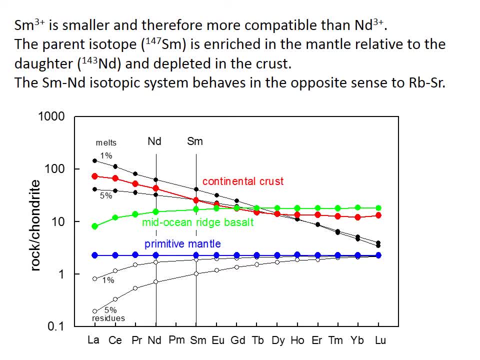 Okay. So if we look now what happens when we melt the mantle, So this is the mantle down here with a chondritic kind of proportion of elements. So if we melt the mantle, if we do a small degree melt, then we kind of move up here. 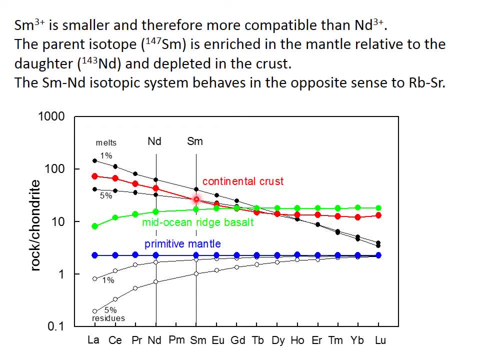 Somewhere into this retina. So in this case, samarium is slightly more compatible than neodymium. So neodymium is enriched in the continental crust, Okay, And what's left behind, kind of the residual mantle, is down here. 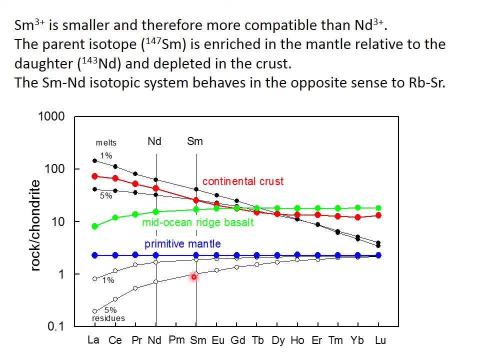 Okay. So we've now depleted the mantle in neodymium, kind of got more samarium in our mantle. Now, when we then melt the mantle again so form a mid-ocean ridge basalt, something like that, that's quite a high degree melt. 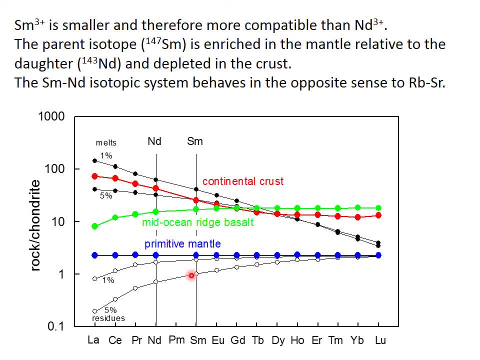 Okay, So you don't fractionate the elements as much with a high degree melt than with a small degree melt. You should have done that with Jeff, So you end up with a mid-ocean ridge kind of still enriched in these trace elements. 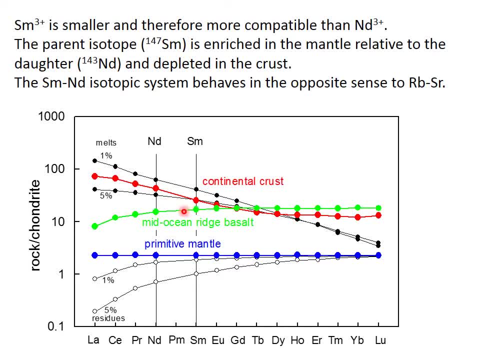 Okay, Because both neodymium and strontium are incompatible, But because we've, we've, just we've, basically we've melted a large degree. melt, the concentration of everything increases by basically the same amount. So what we're looking at now is the continental crust. 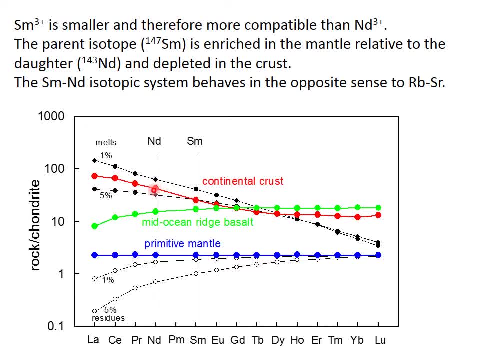 Okay, So we've got a large degree melt. So we've got a large degree melt. We've got less samarium and more neodymium, whereas mid-ocean ridge basalts have got similar amounts of neodymium and samarium. 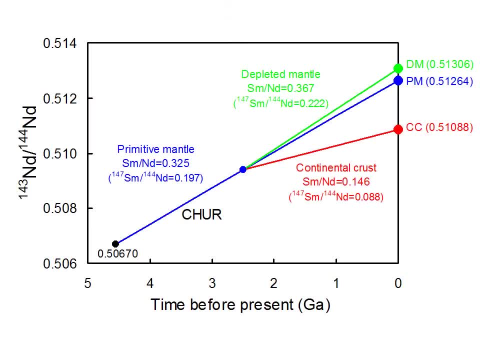 Okay, So over time on the next one, So over time now as we grow in, 143, 144.. So this is so, basically, we've normalized the radiogenic isotope 143, neodymium, to a stable isotope 144. 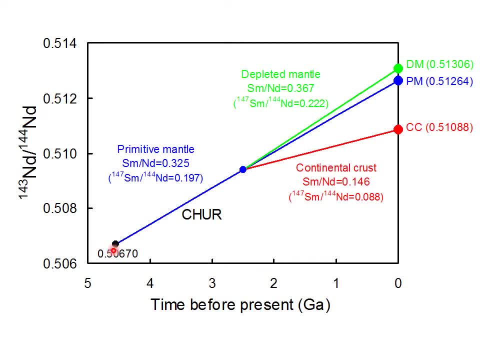 So, once again, okay, we start out at some initial value When the Earth is formed and over time we increase the amount of radiogenic neodymium. Okay, But this time when we form continental crust, okay, we're removing samarium. 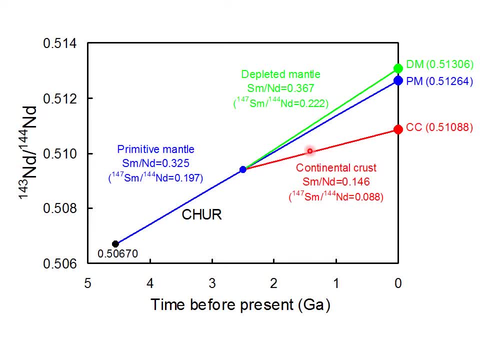 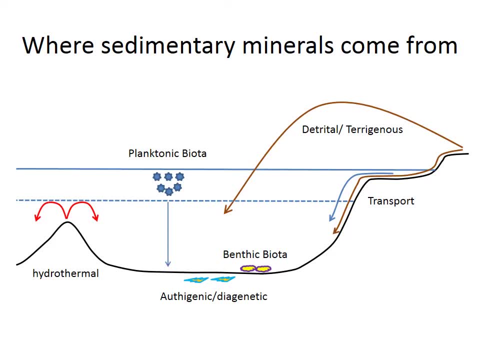 We've got less samarium than we do neodymium, So it evolves at a slower rate along this line, whereas depleted mantle is up here. Okay, So that's. that's just a recap of how radiogenic isotopes work. So now I just want to talk about something that's really important for geochemistry. 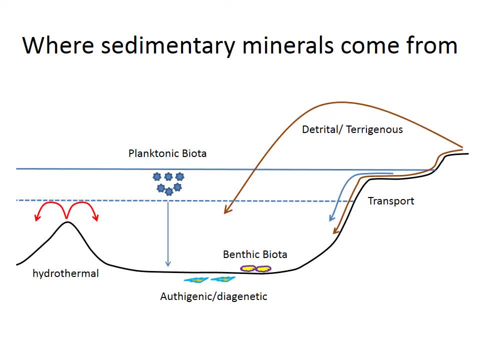 And that is it really matters what you measure. Okay, So if we were to just get some sediment out of the deep ocean, dissolve it all, measure it, we wouldn't really know what that was telling us about the environment in the past. 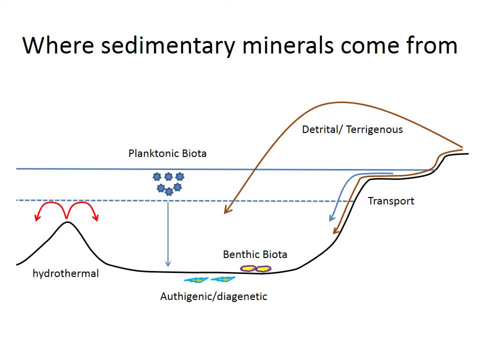 because the components of that sediment come from lots of different places. Okay, So if we wanted to know about the chemistry of the ocean, okay, we would have to isolate a component. We would have to isolate a component of the sediment that was formed in the ocean. 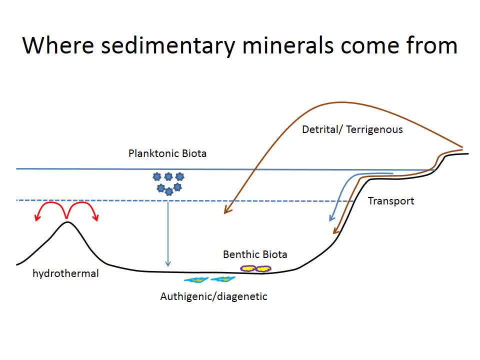 Okay. So, for instance, if we wanted to know about the oxygen-isotope composition of the ocean, we might pick out planktonic forams- okay, that grew in the ocean. Okay, We wouldn't pick out bits of quartz, which also have oxygen in. 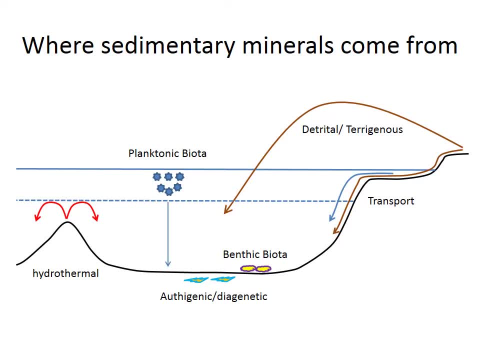 because they'd be telling us about the oxygen-isotope composition of wherever that quartz formed, which would be on the land somewhere, presumably Okay. So there are a whole bunch of ways that that things that are in our sediment can get kind of chemistry. 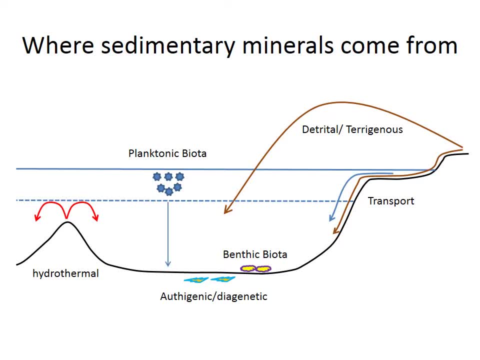 get some goodies in it that we can measure. So things can, things can precipitate in seawater. so things with shells: okay, so they'll record composition of the seawater in the part of the ocean that they formed. Okay, So you might want to be, for instance, with oxygen-isotopes. 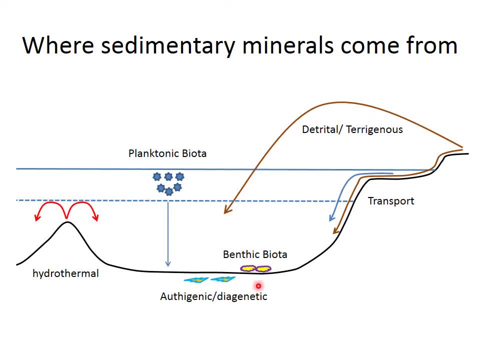 the oxygen-isotopes of the surface ocean and the deep ocean will be different. Okay, So if you wanted to measure those differences, you would measure something that grew in the surface ocean and something that grew in the deep ocean. Okay, There are other inputs of elements of the ocean. 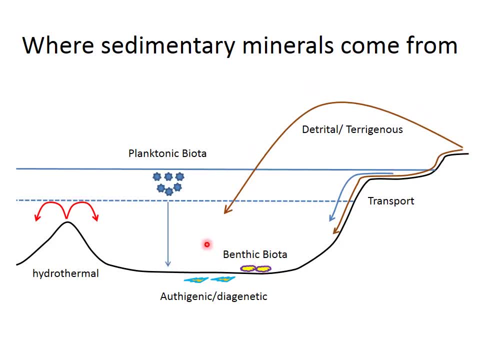 So torriginous, so dust, okay, gets put into the deep ocean. So if we wanted to learn about where that dust was from or how much of it was being inputted, we would try to measure some element, okay that was concentrated in dust, but not concentrated in stuff that's in seawater. 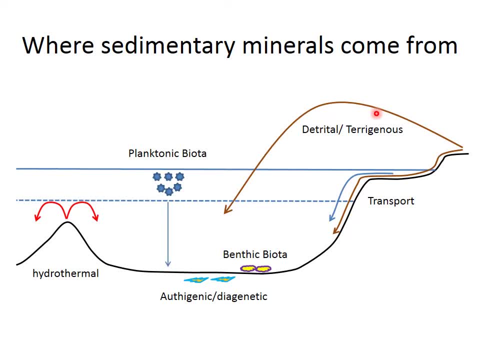 So something maybe like titanium, okay, refractory elements that are in continental material but don't dissolve in seawater, Maybe thorium, things like that. Then you've got other things that basically the coatings on things that are on the seafloor. 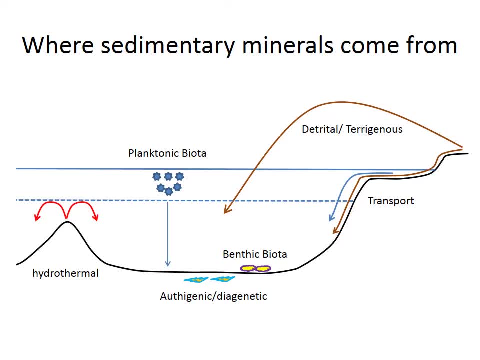 Okay. So sometimes when something is sitting on the seafloor it'll be coated by something, maybe an iron manganese oxide, And that iron manganese oxide will scavenge elements from seawater and we'll see this later on and record the composition of seawater at that site of scavenging. 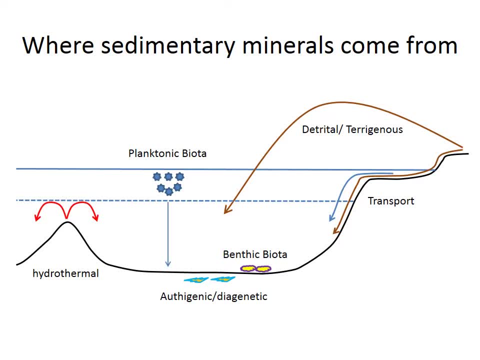 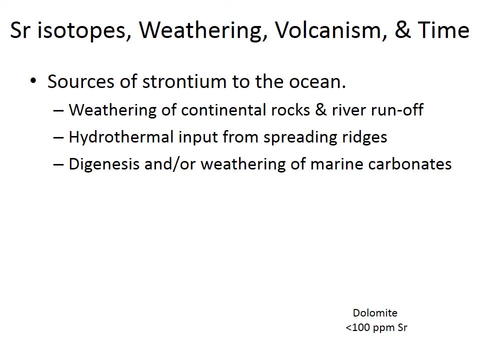 So it's really important to consider where the thing that you are measuring has got its elements. Okay, So just bear that in mind. for the rest, Okay, Okay, So Strontium isotopes. So where does the ocean get its strontium? 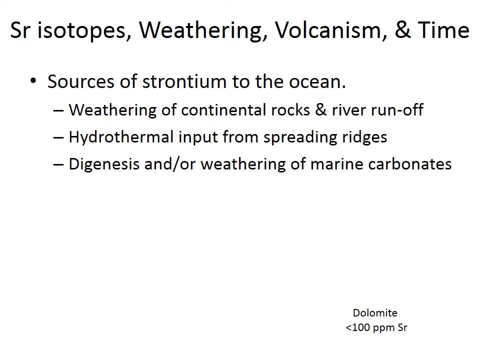 So there are three main sources. So you can weather continental rocks: Okay, That puts strontium into river water That enters the ocean. Okay, You can, strontium can enter through hydrothermal activity with basically volcanic rocks, so mid-ocean ridges. 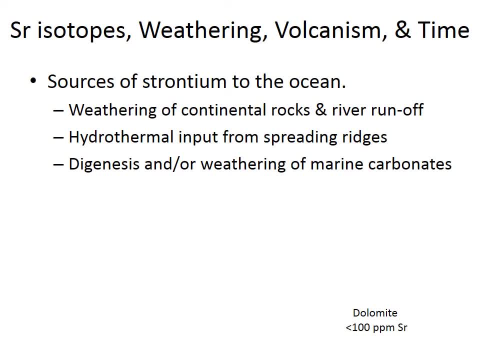 Okay, So that brings in strontium to the oceans. And there's a third term of diagenesis of sediment And that brings a different kind of source of strontium to the ocean. We'll just look at those in turn. 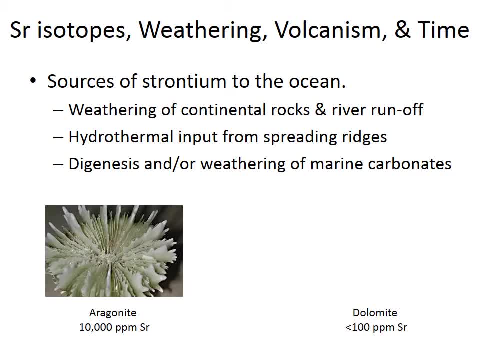 So this is kind of a diagenesis. So this is- I think this is a coral. It's made out of aragonite. It's got loads and loads of strontium in it, because the crystal structure of aragonite allows it to incorporate strontium. 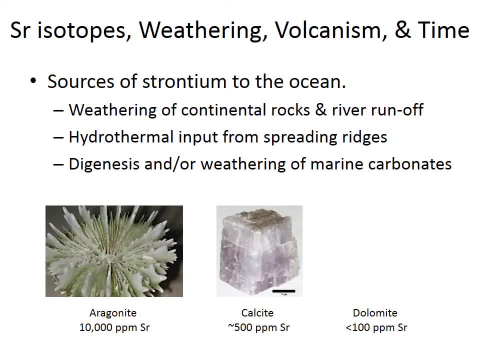 Calcite, much more common in the geological record. That's got a much lower concentration of strontium, as does dolomite. So if we take an aragonitic coral, okay, and over time that might turn into calcite With diagenesis. 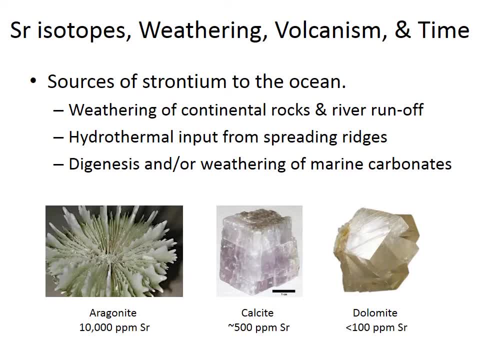 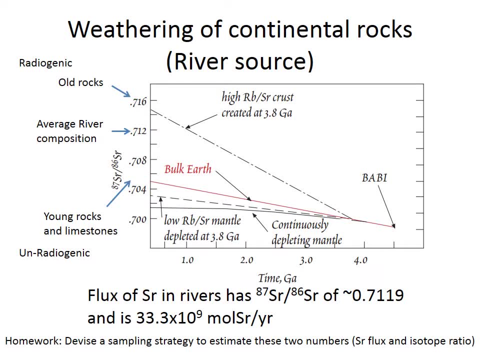 All the strontium that was in the coral will be released into the pore water environment to ultimately go back into the ocean. So just briefly weathering. So we've just discovered why the continental crust will have a high strontium isotope ratio. so on this side now we've got the strontium isotope. 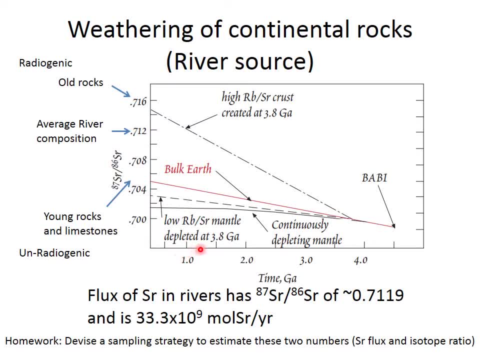 So this is backwards from the once we've seen before. So can't? old continental rocks will have a very high strontium isotope ratio And you could see the quoting here and represent what I've said here. And we've seen that hinting that any of these provincial althey and Aldenbad rocks, flap fish that line with the straxion arsenic may respond to their own strontium ionoten. 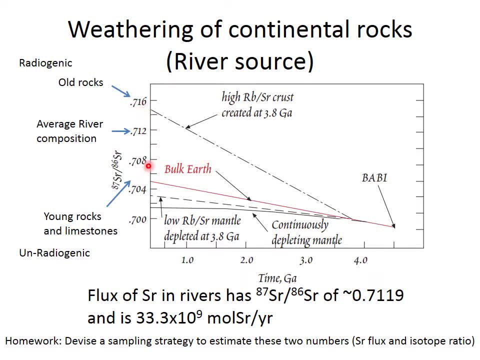 So we'll have a very high strontium ionoten, in the same way as we have in the straxion arsenic in the straxion revenir house strontium isotope ratio. okay, younger continental rocks will have a lower strontium isotope ratio. 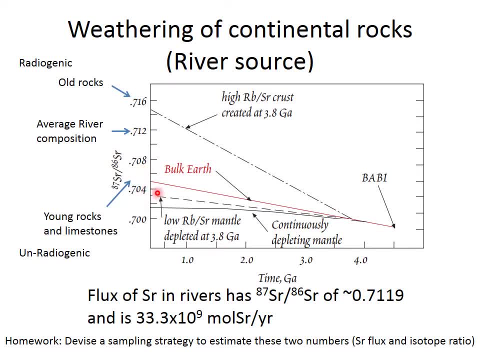 and stuff that comes from like volcanic rocks, that comes from the mantle, will have a very low strontium isotope ratio. so, um, if you the weathering source is probably somewhere along this axis, here, somewhere up here, kind of average river composition, okay, that inputs into the ocean. 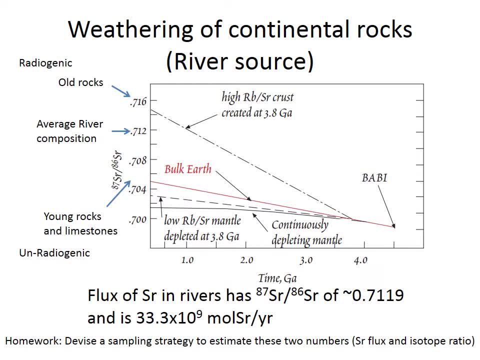 strontium with a specific isotope ratio. okay, and you can see down there there's the um i've put on the. the average ratio is 0.7119, something like that um, and it's quite a large flux: 33 times 10 to the 9 moles per year. so that's gigamoles, which is a huge amount um. so you might. 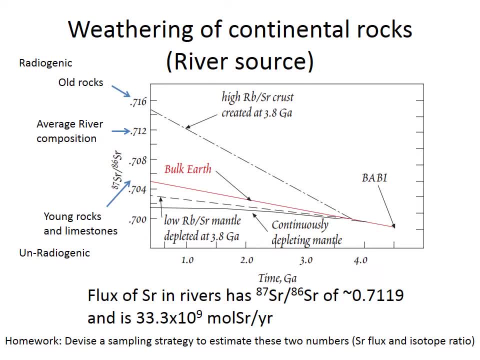 want to think about how you might get those numbers. if you, if you were a, if you were a scientist and you wanted to know how much strontium was going into the ocean from rivers and what its isotope ratio was, how would you work out those two numbers? okay, how would you go about measuring? 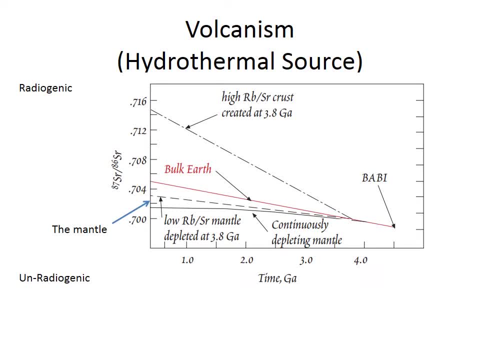 those. come on, talk about that and um, so the hydrothermal source. so this is stuff that's coming basically from the mantle. okay, the mantle will have a very low strontium isotope ratio because over time it's had a very low rubidium strontium ratio, um. so you might have seen this diagram before in, i think, ele. 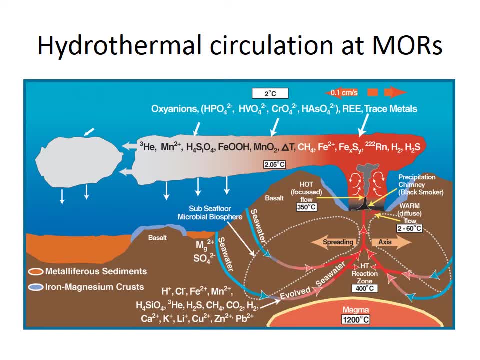 or something like that. but this is basically just a cartoon of we have seawater gets sucked in to hydrothermal systems, um that mid-ocean ridges, because once the water is poor, water is basically in the rock. it heats up, expands and rises out the top. so you must be circulating water through the system. um so, uh, strontium gets. 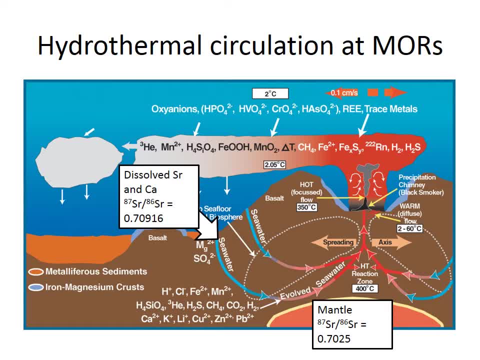 sucked into this system from uh, from seawater. so the water as it goes into the system starts out with some strontium in it, okay, and then it passes through the uh, passes through the rocks, and those rocks have strontium in them. that's basically from the mantle. so we'll have a very low strontium. 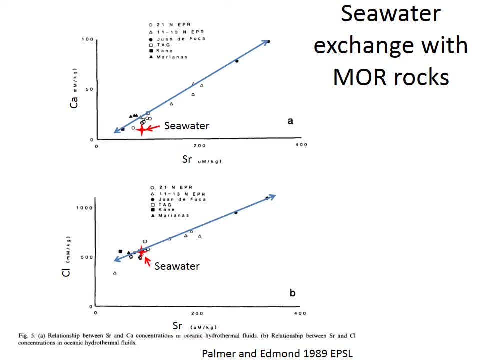 isotope composition and if we just look at what's happening. so this is: these are measurements of water at hydrothermal vents. okay, so we're looking at basically the concentration of strontium along the x-axis and then, on the vertical axis, looking at the concentration of calcium and the concentration. 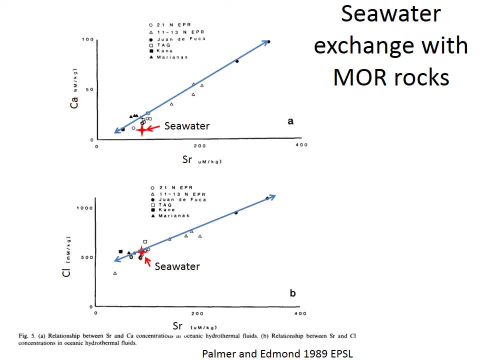 of chlorine and because we've got this very, very kind of like tight correlation between the two. okay, this: this tells us that there's a very high concentration of strontium along the x-axis and exchange of strontium and calcium between seawater and rocks. okay so, because the correlation is so. 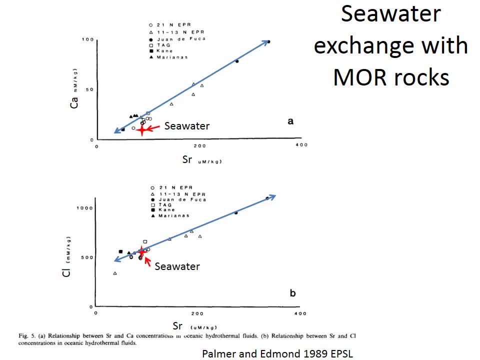 good. this basically tells us that, because calcium and strontium, we'd expect to behave quite similarly anyway, because they're very close to each other in the periodic table in the same period. okay, just one above the other. so what's happening here is we're basically exchanging strontium from seawater. 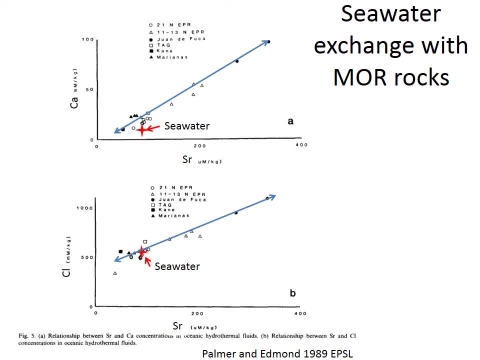 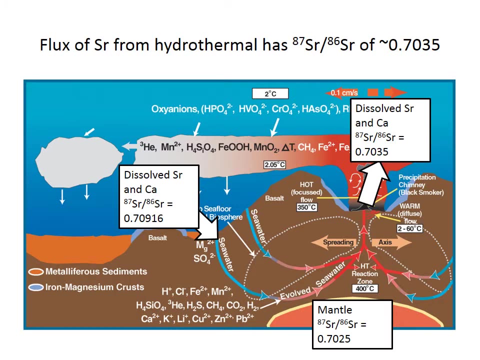 with minerals in the um, in the crust, i guess, um, so minerals that contain calcium and strontium, and we're basically just swapping the strontium backwards and forwards. so when we look at what actually comes out of the uh, of these hydrothermal vents, the strontium isotope composition here is some intermediate between 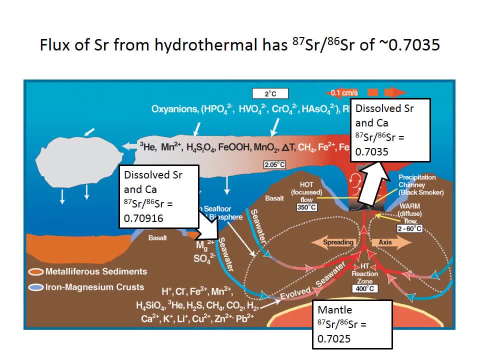 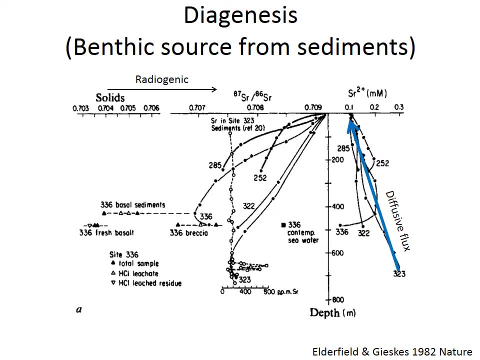 seawater and, uh, the mantle source here. okay, but you can see it is much lower than the seawater composition. it's much lower than the weathering flux, which was point seven, one, one, nine, something, okay, so the last, uh, the last source is this flux from sediments. 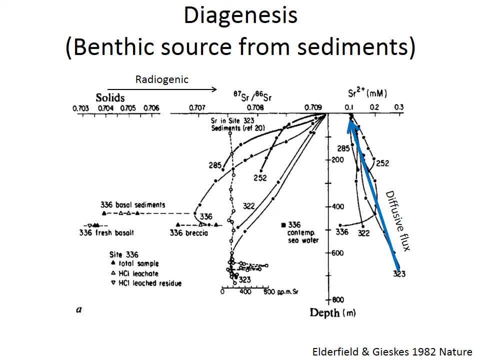 so this is a composite plot of uh measurements from down deep drill cores into into the into ocean sediments. okay, so you can see here that they've. they've drilled down maybe 800 meters into the sediments and they've measured the concentration, an isotopic composition of the 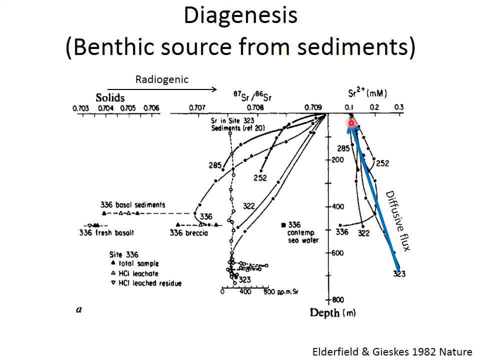 pore water, so the water in between all the grains, and you can see here that there's a. the concentration increases with depth. okay, so if you have a concentration gradient, that much means that there must be diffusion along that gradient. okay, stuff diffuses from high concentration to low concentration. so this: 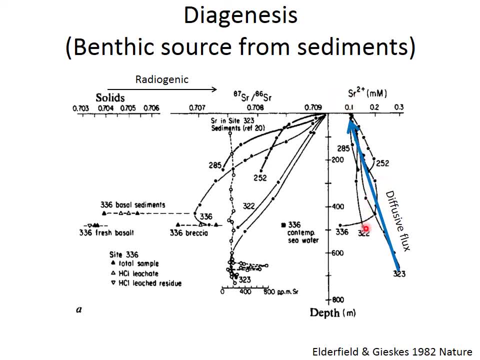 concentration gradient is telling us that there must be a flux of strontium from the sediment into the seawater. okay, so we can. we can actually, by some diffusion modeling, we can work out what that rate is. okay, we can extrapolate that over the whole ocean, because sediment is pretty much the same. 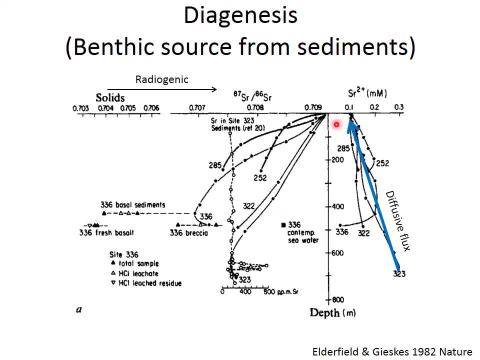 everywhere in the deep ocean and then if we look at what isotope ratio that sediment is or that poor water is, we can see that all of the- so these are profiles of this, of the profiles of the strontium icons- take composition. so seawater is up here and as you go deeper and 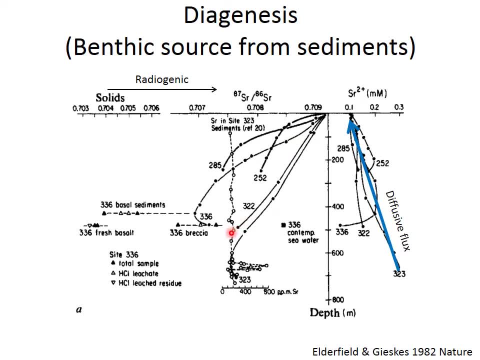 deeper into the sediments as more and more stuff is being dissolved and being put into the water. we can see we get lower and lower strontium isotope values. point seven, nine, seven, one, five. So this is a mixture of dissolution of calcium carbonate, which is from seawater. okay, 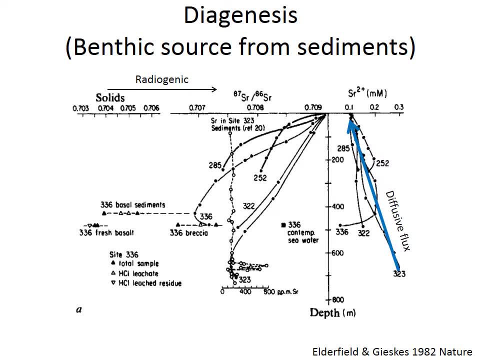 Which. so the seawater composition of strontium is quite complicated. It changes through time, but it doesn't change by much. So it's this modern seawater is up there. This point down here is where seawater, the composition of seawater at the time the sediment was deposited. 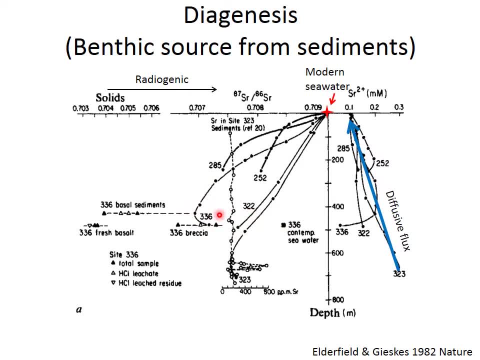 So because all of the pore water values are lower in their strontium isotope composition, that must mean we must be adding strontium from something that's not carbonate produced from seawater, And what that is is basically small, very small amounts of volcanic ash that are in the sediment. 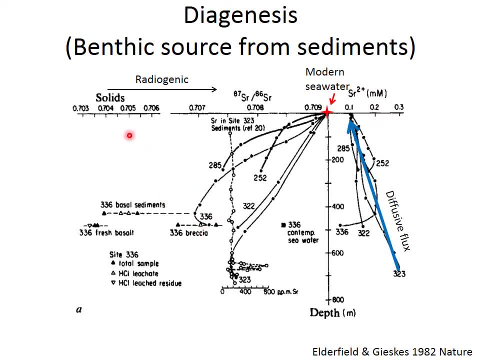 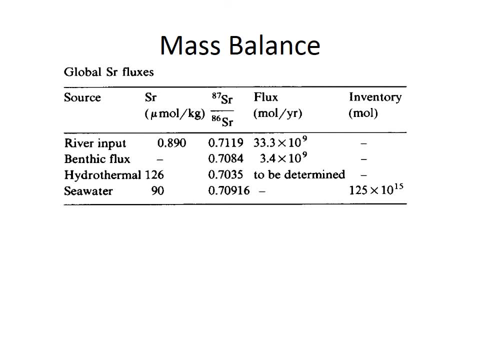 that dissolves and releases its strontium and that has a very low strontium isotope composition. So just to summarise that, okay, we've got different inputs. We've got the river inputs, the benthic flux, which is from sediment. 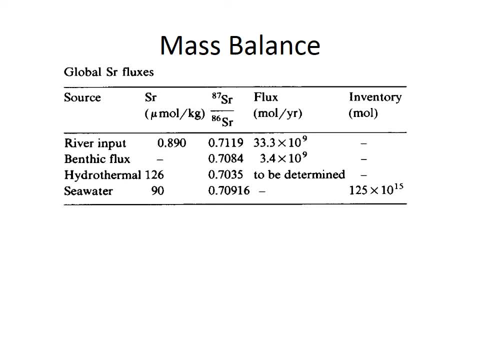 and the hydrothermal influx: okay, And we can put numbers on those for what the strontium isotope ratio was or is from those. okay. And for the river input and the benthic flux, we can kind of work out what the flux is okay. 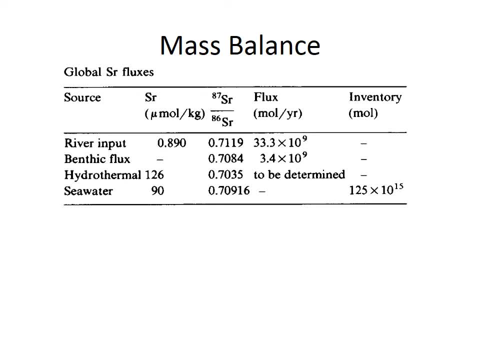 And the hydrothermal flux. we can also work that out because we know, basically we've got six unknowns. well, one unknown six. We've got enough knowns and unknowns to work out what it is and we'll do that in the practical. 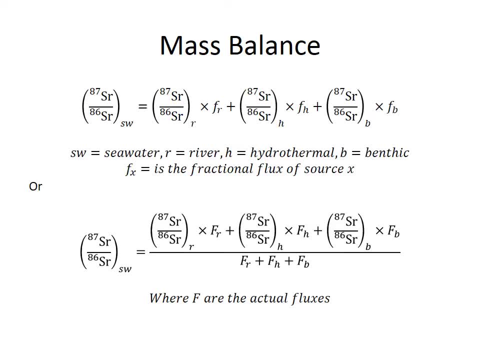 Okay. so the way that we go about doing that is, we can use this concept of mass balance. So this is very simply- I mean it's very similar to mixing paint. So if you imagine you had kind of white paint and black paint and you mix those together, okay, 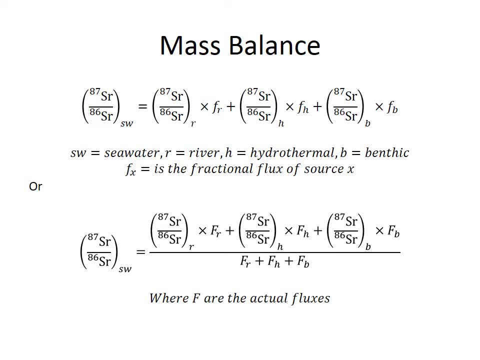 the final colour that your paint is or the shade of grey it is. I'll resist the shade of grey. The shade of grey that your paint is is a function of the proportions, of the different amounts of paint you've had, and like how black and how white the paint was. 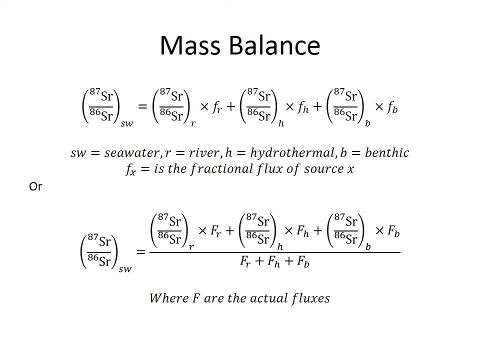 So in this case we've got. so, for instance, here we've got the strontium isotope. composition of seawater is a function of the compositions of the river flux, the hydrothermal flux and the benthic flux, basically, each of those times, by the relative importance of each of those fluxes. 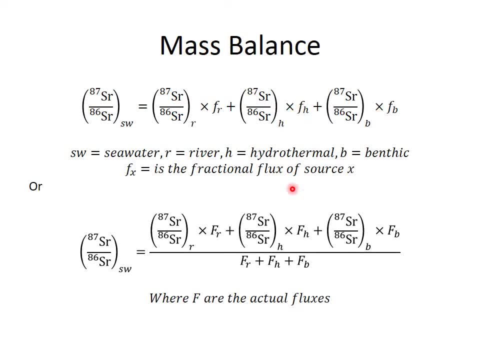 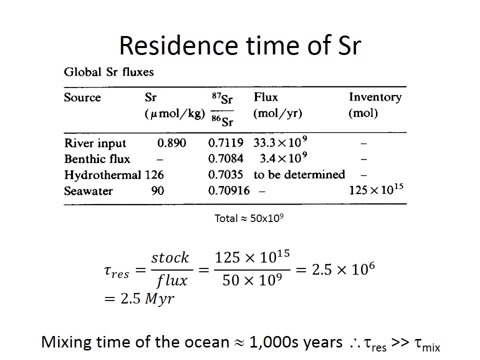 So these are the fractional fluxes, okay, So we can convert those into real fluxes by dividing by real fluxes. yeah, and we'll do that in the practical. Okay, so that, yeah, that homework exercise will basically seem practical. 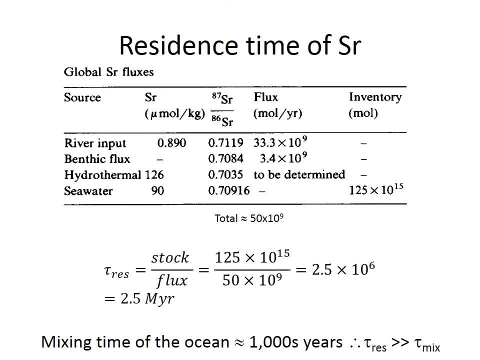 Now the thing about strontium in the ocean is that we can- we can. if we're gonna measure the isotope composition of something somewhere in the ocean. we want to know: is that representative of the whole ocean or is it just another unit? okay, 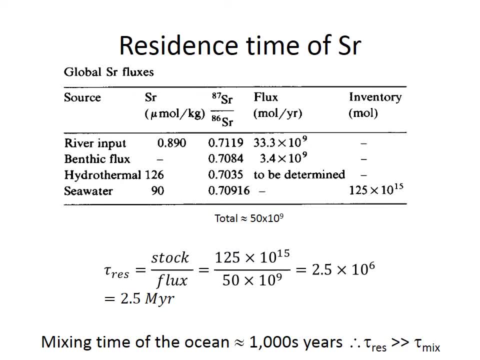 just representative of that bit of the ocean that we've measured. So for instance, with oxygen isotopes each part of the ocean will have a slightly different oxygen isotope composition because the oxygen isotopes scale well with salinity. you should remember from the practical Now. that means that if you measure the oxygen isotopes, 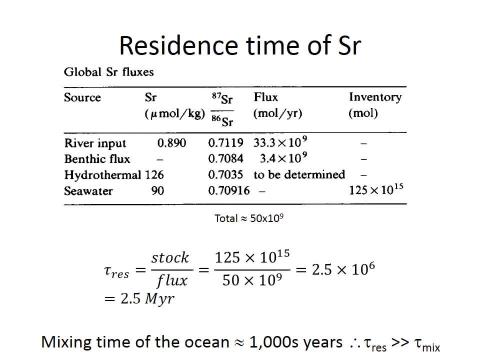 in one place, that's not necessarily representative of the whole ocean. Whereas with strontium we can calculate the residence time from the data here. So we know how much strontium there is in the ocean by working out basically the size of the ocean and measuring the concentration. 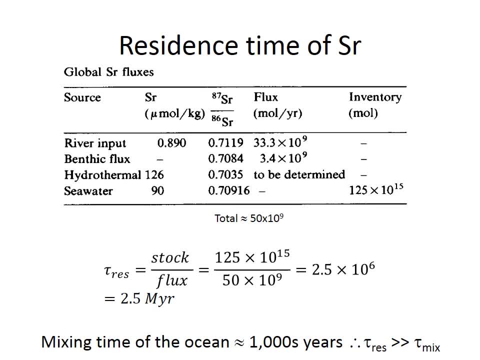 And we can work out what the flux is, So what the rate of input is, And from that you can work out the residence time, which you should have done in previous courses. But basically the residence time of strontium is two and a half million years, So that means that if you change the fluxes, 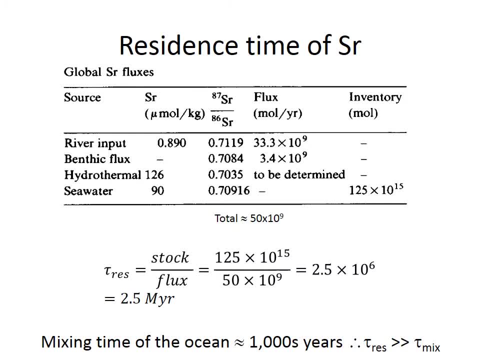 if you halve the flux, it would take two and a half million years for the concentration to change by half. Okay, So the concentration changes very slowly in the ocean. Okay, And you can see, the mixing time of the ocean is very short of the order of a. 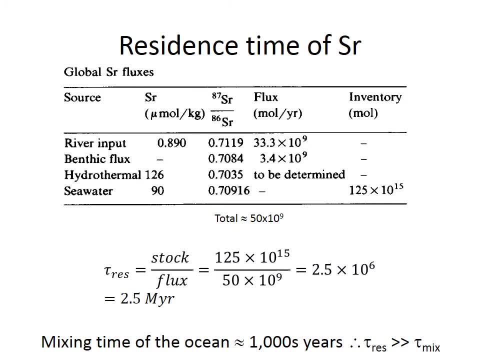 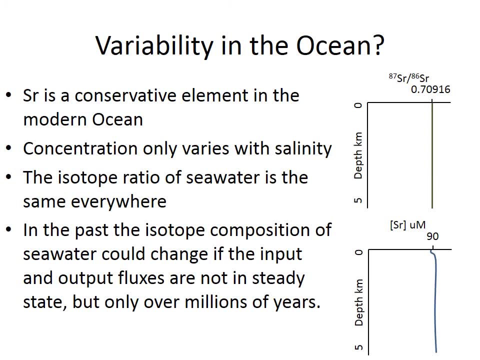 thousand years. So that means that because the residence time is much longer than the mixing time, everywhere in the ocean has the same strontium isotope composition. Okay, So that I mean also means that the concentration is basically only varies with salinity. 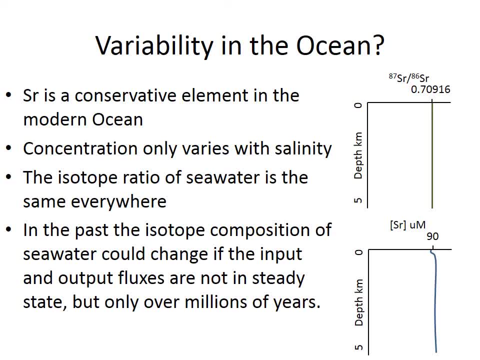 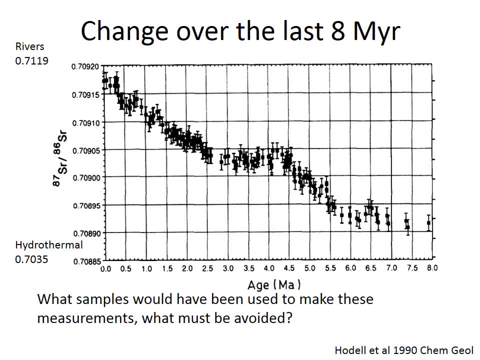 Okay, So this is. this is quite, quite neat because this: this means that we can measure the strontium isotope composition in one place in the ocean and that will tell us about the strontium isotope composition everywhere in the ocean. Okay, So this is some. 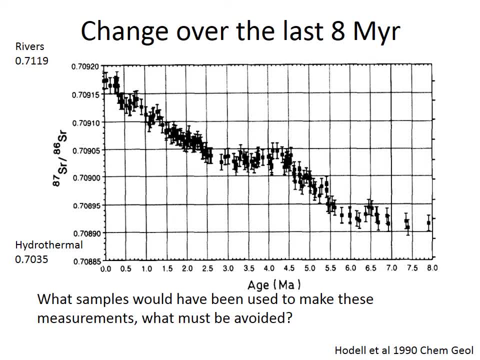 these are sorry. these are some data- It's a bit old now, It's like 25 years old- Of strontium isotope measurements, of something that represents the ocean. So I think these were measured on a four-ammoniferous. Okay, So they precipitate in the ocean. So 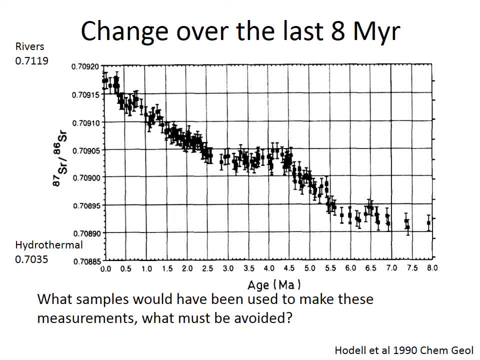 they've taken strontium from the ocean and we can then kind of infer that this is the strontium isotope composition of the ocean. So we can see here that this is the, this here is the, the composition of the ocean now and back through time. 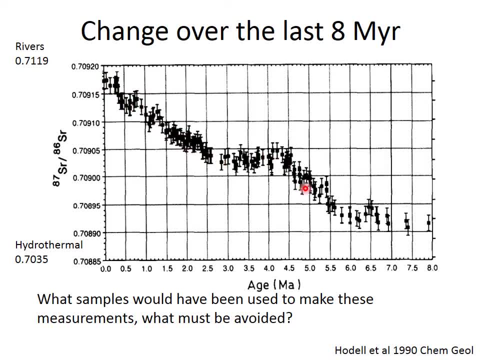 it changed, Okay, Okay, But it's changing quite slowly. So we've got a scale here of many eight million years, Okay, And you can see. so the river influx is point seven one nine, So that's way off the scale at the top here. 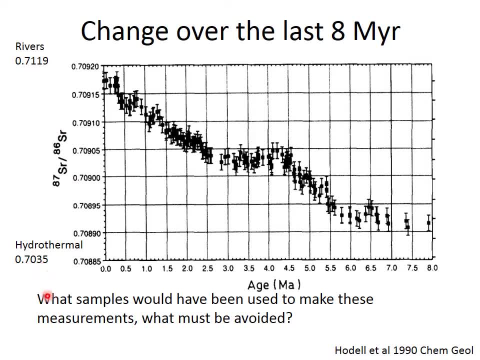 Hydrothermal flux, point seven, three, five. That's way off the scale down the bottom. Okay, So we're actually changing the isotopic composition by actually relatively small amounts relative to the compositions of the fluxes. Okay, So some questions you might want to ask yourself is: what kind of things? 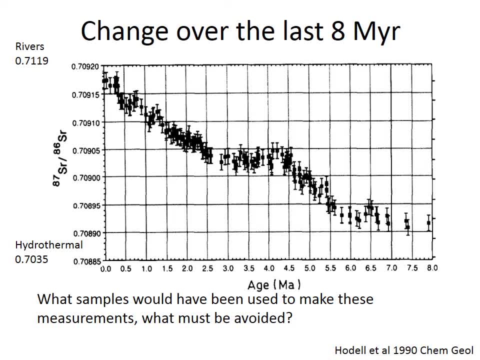 were we measuring and what? what do we need to avoid when we're measuring the thing? So I've said these are measured on four ams, But would that be an appropriate thing to measure back through all of geological time? Anybody into paleontology? Okay, So four ams haven't been around that long, So it's. 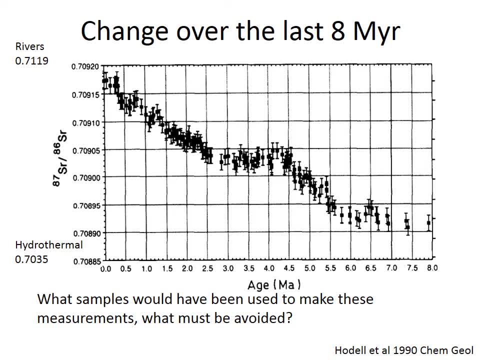 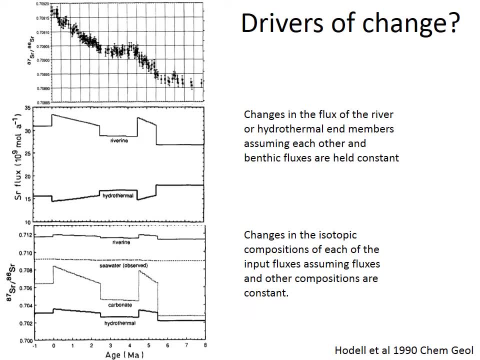 not, you can't measure from the whole geological time. Okay, So what's driving these changes? Okay, So we know that the current fluxes and isotopic compositions that are going in from rivers and hydrothermal and the benthic fluxes, 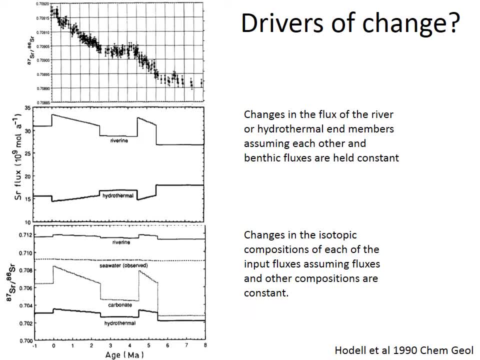 So it's very unlikely that the benthic flux will change. Okay, Because that's basically the bottom of the ocean and conditions at the bottom of the ocean are fairly stable. But we can change the composition of the ocean by changing either the magnitude of the flux, 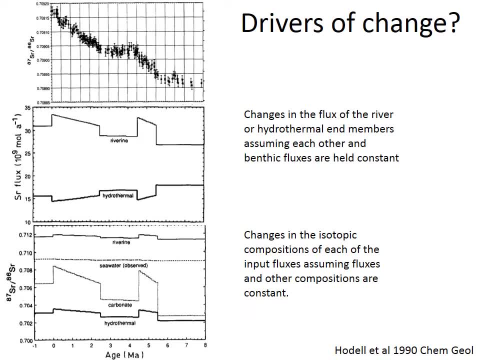 So if we start adding more riverine strontium in, that should make the isotope ratio go higher- Yeah, Because that's got a more radiogenic, so a higher strontium 87, 86 ratio. Or if we increase the hydrothermal flux, if we made mid-ocean ridges hotter and spread more fast. 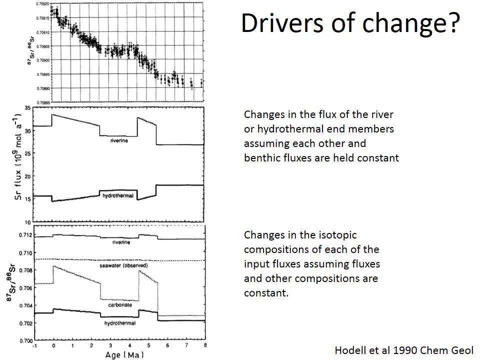 that would bring more strontium in With a low strontium isotope composition. So we could change the fluxes or okay, or we could actually change the composition of the end members. So if rivers started having a different flux, if we started weathering older rocks or younger rocks, that might change the 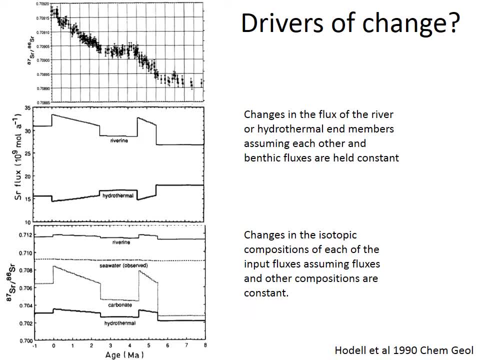 end member composition. So that would change the strontium isotopes through time. So just a example, This is basically. these are model examples of what happens So if we change the strontium isotopes through time. So I've simplified the strontium isotope curve to this, this green line along the top, and then the next figure is basically what you would have to do to reconstruct that green line. 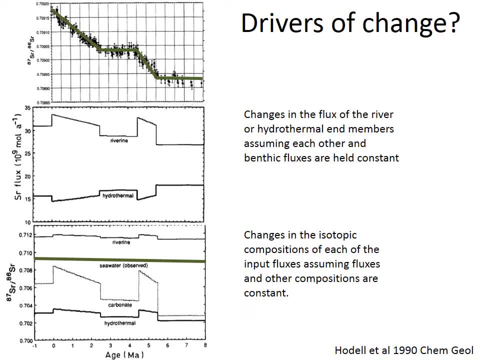 Okay, so the first, the middle panel there is just changing the flux. So if you kept everything else the same and just changed the river flux, that top line which shows that to get the increases where the strontium isotope ratio of the ocean increases, 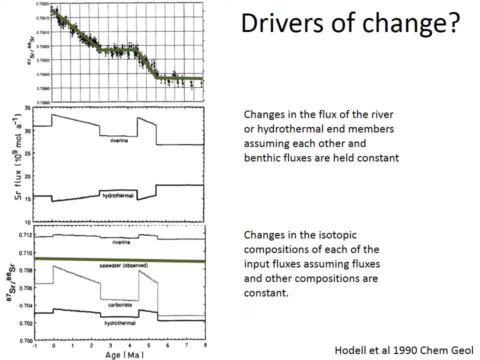 you'd have to have a higher river flux, okay, Or you could have reduced the hydrothermal flux, Or you could change the composition of the fluxes and that's what the bottom figure's doing. And on the bottom figure you can see the composition of seawater is basically that green line is the same green line as on the top figure. 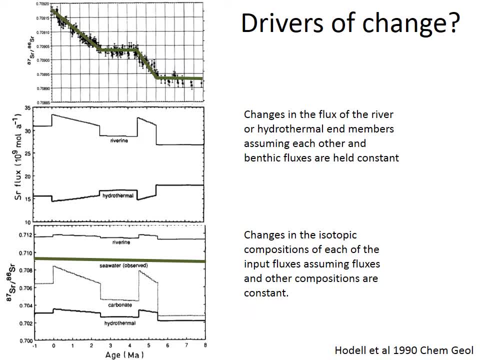 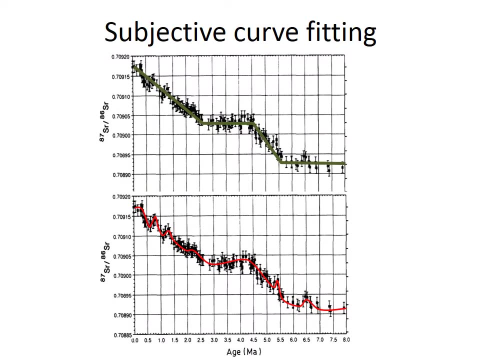 Okay, so you can see that the relative scales are very, very different. So the end, the changing the isotope ratio of seawater is actually quite sensitive to changing the composition of the end members because they're so different. Okay, I just thought I'd put this, this, this, in to give you a little um, a word of caution when interpreting data. 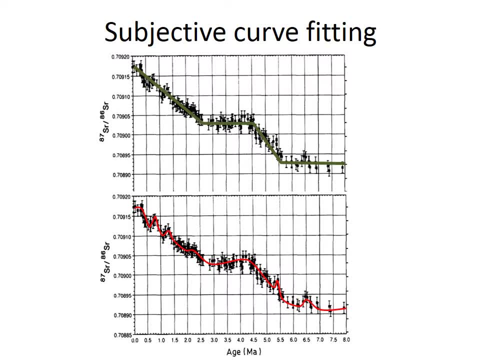 So, uh, so these coloured lines weren't in the original paper, so I've just copied the same figure one top of the other and I've just put through different ways of interpreting that data or those data. sorry, So it's the same thing. so you could say that actually, during this period here there's nothing really happening at all. 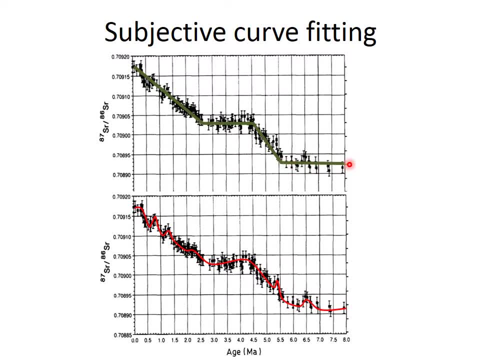 You could draw a straight line through all of those error bars on those data. there nothing happens. Okay, then there's a constant rate of increase, Whereas if you kind of wanted to interpret every little wiggle and jiggle in your data, you could actually say: oh well, there's a, there's an anomaly here. that might be a little pulse of weathering or a changing source of weathering in there. 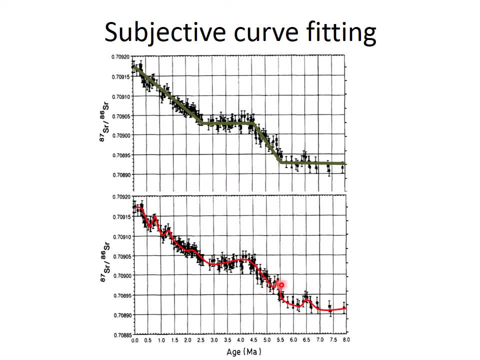 And then you have a gradual increase. There's also these short little pulses of change here. So just just uh, I mean it's. it's one of the things that with quite a lot of geoscience data is it can be quite subjective what you actually interpret from kind of a cloud of data points. 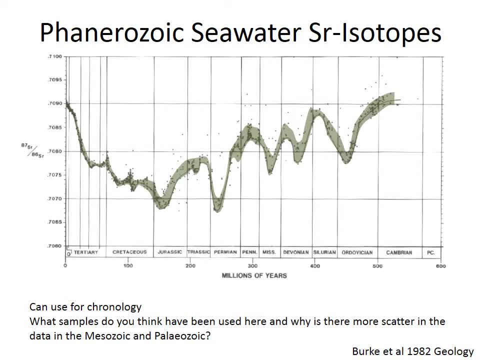 Um, okay, so we're going to actually come and use this now and see what- what we can do with it. So this is uh. so I've basically now expanded the the age scale and now we're looking across the whole of the Phanerozoic. 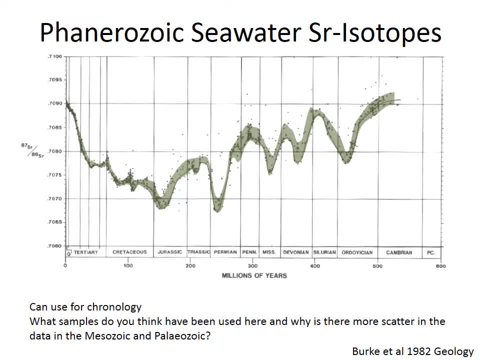 And we can see here how the strontium isotope composition of the ocean has changed through time. Okay, Um, you can see that the the scatter of the data gets bigger as we move back in time. Okay, And we'll we'll have a look at why that might be and what we can do about that. 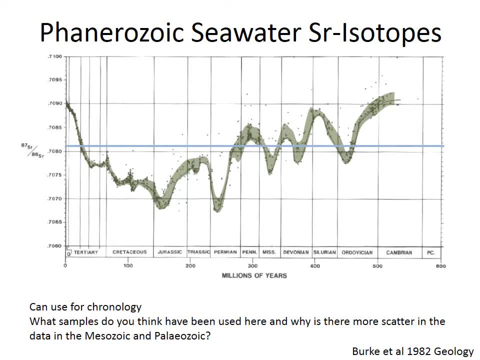 Um, okay, so we can we start thinking if we, if we measure the strontium isotope composition of something that we find in some sediment, Okay, And we know we had these data beforehand, We know that these, uh uh, the age of that sample must have been lower. 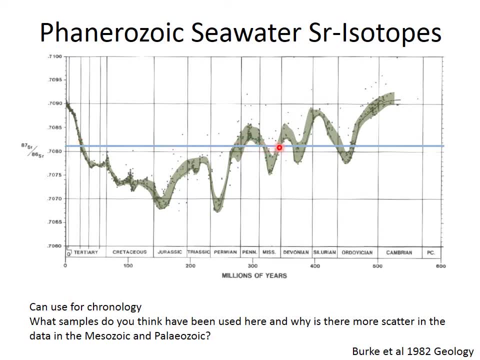 Okay, must be either at this point, somewhere over here, somewhere over here, somewhere over here to here, or here or here. Okay, So we can use it to- to basically try and narrow down how old we think something is. So we-, we-, if we- if we knew that our sediment was. 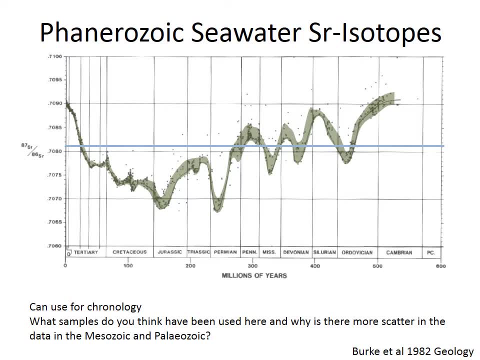 you know from the tertiary, then we could know exactly how old it is in this class and we could ignore those older bits of the curves. But it does get a little bit more intelligent than that. So- so for this size, if we know that it's. 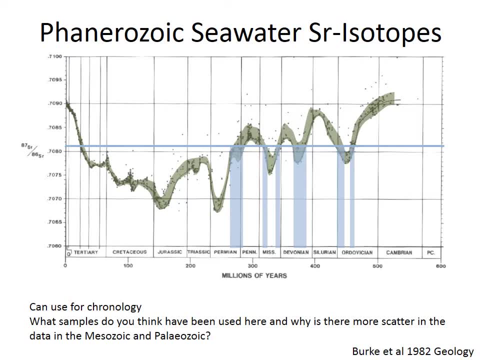 kind of actually from the um- Paleozoic um- we say, well, it's- it's one of those dates. Okay, Not much use. But if we then look at our um, where our sample is stratigraphically, 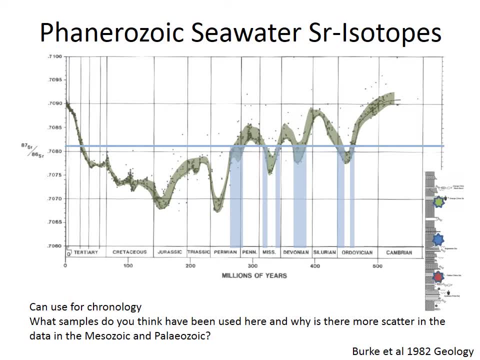 so we say we've de- we've measured it from- from there. and then we measure some other samples above and below. we know that the green one must be younger than the blue one, which must be younger than the red one. Okay, Because they're one on top of the other. 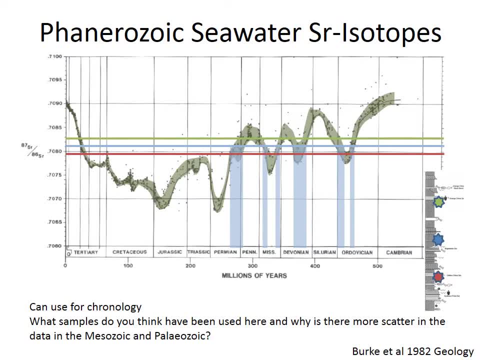 That's how geology works. Okay, So those are the ages now. Well, those are the strontium isotopes, say we- we measured. Okay, So we know now that say, for instance: those are now the only two ages that that set- that can be. 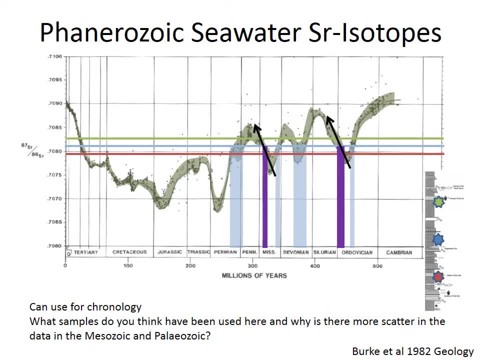 because those are the only points where the um, the thing is increasing. Okay In age, Okay, So we can- we can- start to use it as a chronological tool, Um, but when we do that, we need to worry about some of this scatter. 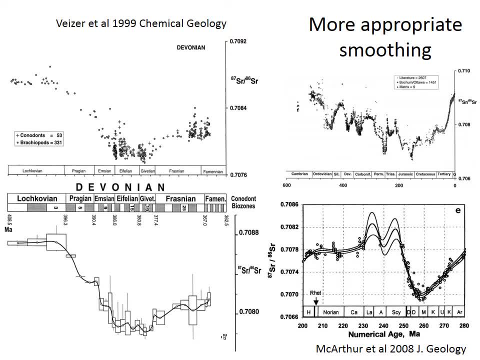 Okay, And we want, ideally, because we know that the residence time of strontium is quite long. Okay, That means that at any one time, all of the ocean must have the same strontium isotope composition. Okay, So this, this scatter here. 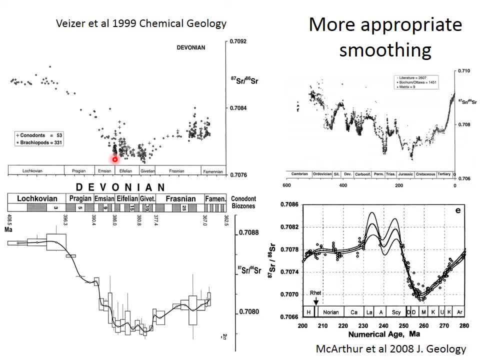 okay, cannot be real. Okay, This must represent some error in either our measurement or bias in sampling. Okay, Because seawater at any one time can only be one value. Okay, So you can take all kinds of approaches to this kind of thing. 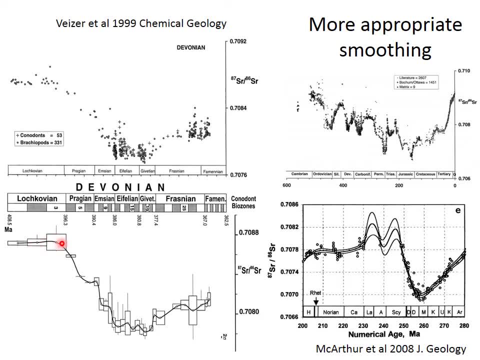 So you can- this is something some people like to kind of like group their data together into little boxes and then kind of work out what the spread is and use that as a kind of like a smooth curve. So this line going through here is not is basically is an overestimate of your confidence in what the actual value of the ocean is. 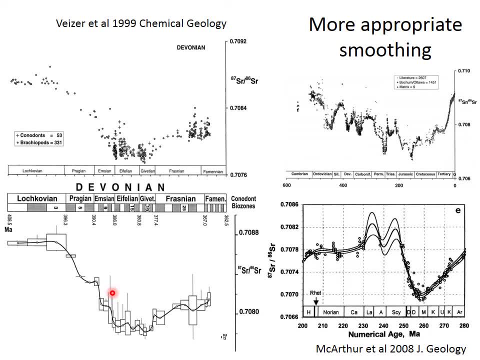 Because some places there's there are big errors, Okay. So maybe something more appropriate might be something like this, where you actually get some realistic estimate of the, the uncertainty. So for instance, here this point, here there's only one point that they've measured. 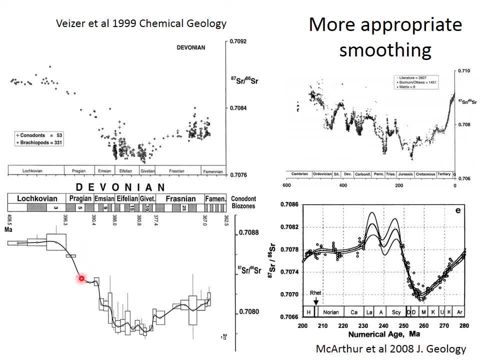 And they've said on this one: oh, that gives us really small error, Okay, Which is obviously a ludicrous statement, Okay, Whereas over this approach here, where there is very little data, they tend to have quite large uncertainties, which is more appropriate. 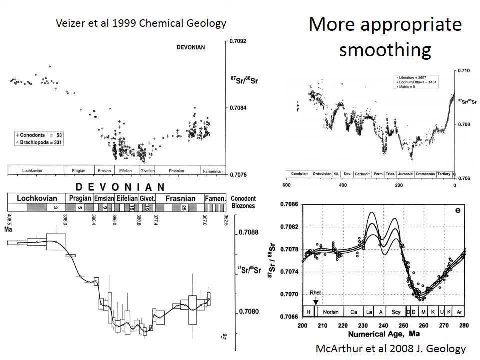 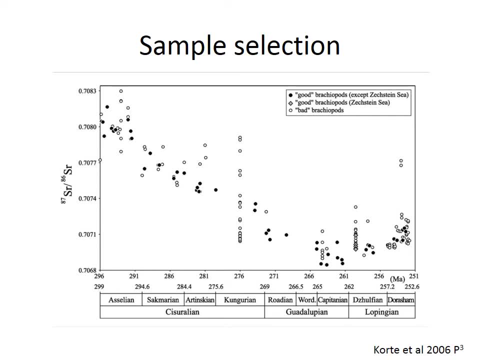 So you've got to think quite carefully about How you smooth your data between points, And I just did a little thing about sample selection. So again, these data in the middle here we know that they're all the same age. Okay, We might even say that they were all sampled from the same bed, in a, in a geological formation. 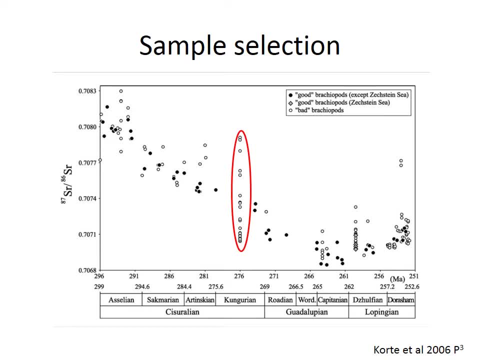 So they must be the same age And we know that they cannot all have different strontium isotope ratios Because the mixing time the ocean is too short relative to the strontium, the residence time Of strontium. So that means that there must be something going wrong here. 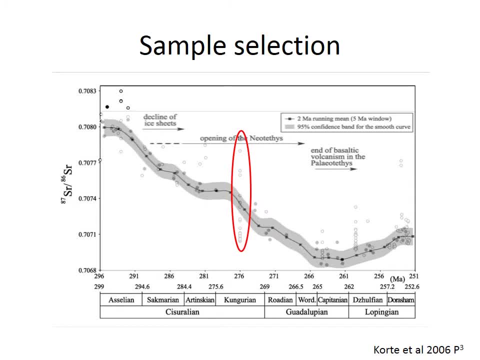 Okay, So what these people have done is they've basically they've divided their samples into good samples and bad samples. Okay, The good samples are the one with the solid little circles, The bad samples are the ones with the open circles, And they've just used the good samples to figure out what the seawater was over time. 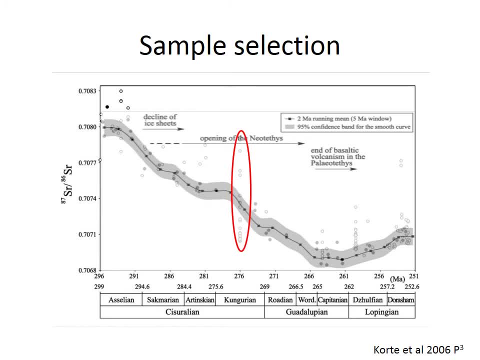 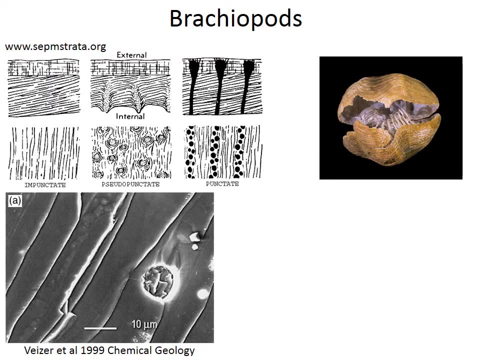 And that's given a fairly good result. Now they haven't just chosen that, you know. oh, I quite like these ones and I don't like these ones for no reason. So they've actually, that curve is based on brachiopod measurements. 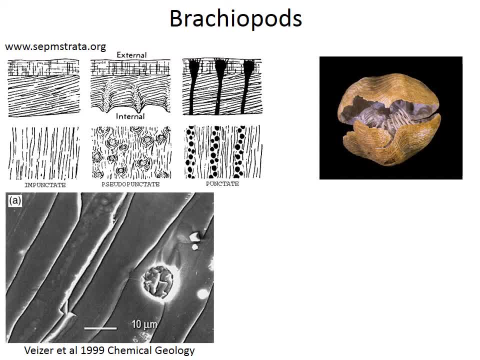 This is a picture of brachiopod, And different types of brachiopod have subtly different structures of the calcite that makes up their shells, And in this case there's this thing called punctuate, impunctuate, Which is basically: does the shell have these little holes running through it? 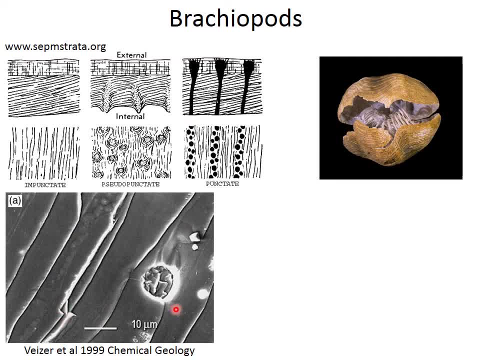 Okay, Now this is an SEM picture of a fossil brachiopod, And here's one of those holes, And you can see that it's been infiltrated. It's been filled with blocky, a blocky mineral. Okay, So that should be a hole. 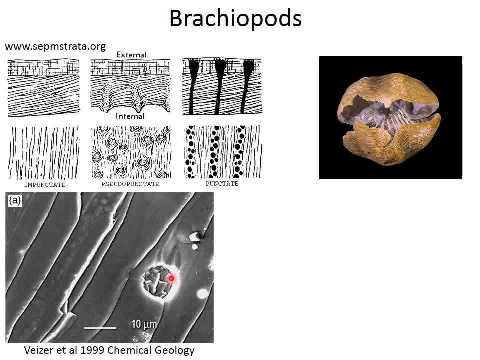 And it's now got something in it that is not a hole. So, since this thing was living, okay, it's died. And as it's been turned into a fossil, some calcite has been added to it. Okay, That calcite will have a strontium isotope composition that is not of the composition of the seawater from which it was precipitated. 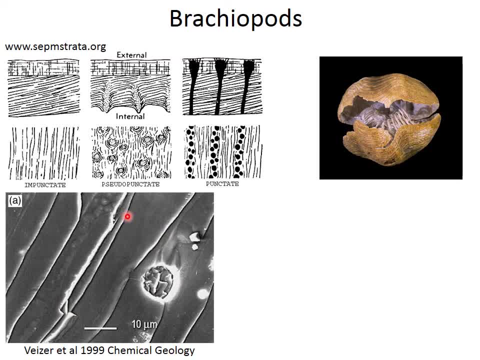 Okay, Which means that if you measured all of this thing, then you would get the wrong number, Okay, So what these guys have done is they've basically they've selected only these kind of brachiopods that don't have holes in. 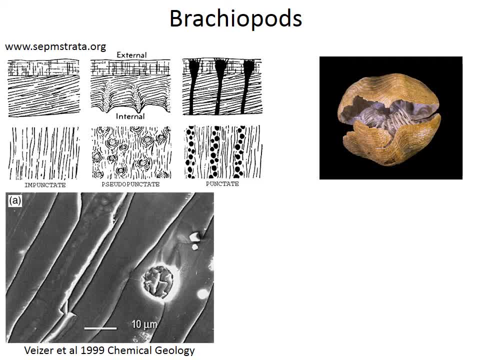 Okay, So they're less susceptible to this kind of alteration. Okay, So that's important as well. So you need to make sure that your sample really is, you know, a nice, pristine kind of representation of the past ocean before you make an interpretation that it is. 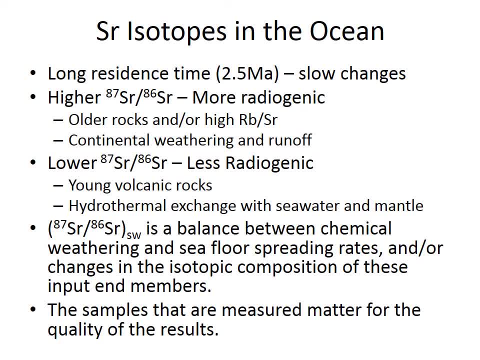 Okay, So to summarize the strontium isotopes in the ocean- and this will form part of the practical as well. So very slow You can go through the reasons why strontium isotopes is higher in old continental rocks. it's lower in volcanic sources. 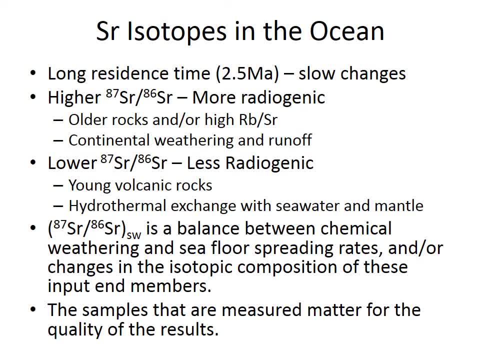 And the strontium isotope composition of seawater is basically a balance between the weathering flux and the hydrothermal flux. So we can use the strontium isotope curve to reconstruct how much weathering there was in the past versus how much kind of volcanism there was in the past. 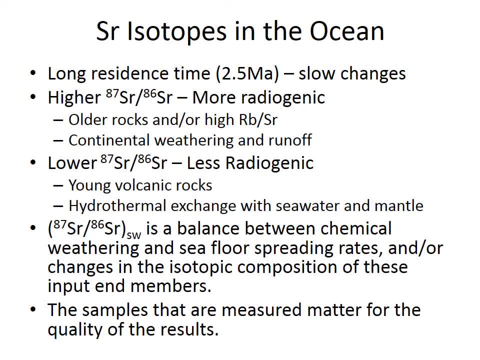 Which is really important, because volcanism adds CO2. To the environment, whereas weathering removes CO2 from the environment. So the strontium isotope curve through time is an important part of understanding the past carbon cycle. Okay, And there's a bunch of reading. 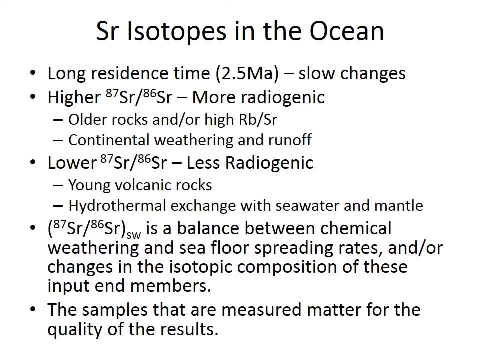 And there's in fact I've put on Learn. there's two papers, one by Peter Molnar and Philip England and another paper by Maureen Ramo and Bill Ruddyman, And they go through kind of the arguments about how strontium isotopes are used to reconstruct. 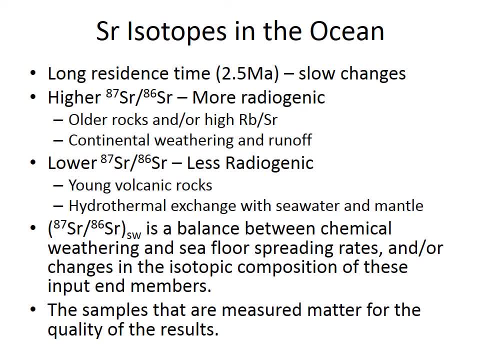 What are the drivers for climate change? So what causes CO2 to change over long geological time scales? And those two papers are really, really quite excellent. They're written by some of the like the biggest cheeses in geoscience. They have thousands of citations each. 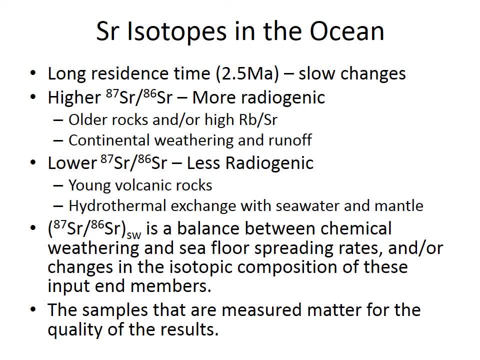 Just for those papers. I mean, they've got hundreds of thousands of citations for all of the scientists, But anyway. so I recommend that, if you're going to read any of the additional reading that I've put online, read those two papers. 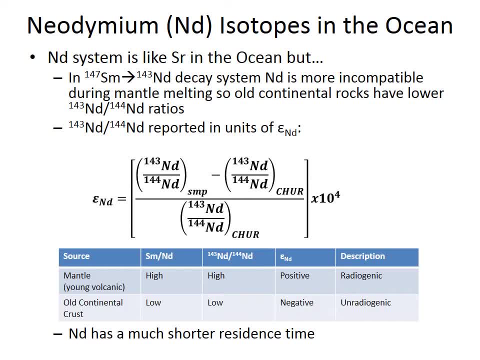 So neodymium isotopes, similar to Strontium, work the other way around. So this equation here is very similar to the delta equation for oxygen isotopes. Okay, we've got the sample. Okay, this is some standard that represents basically what the average, like the bulk Earth, is at the moment. 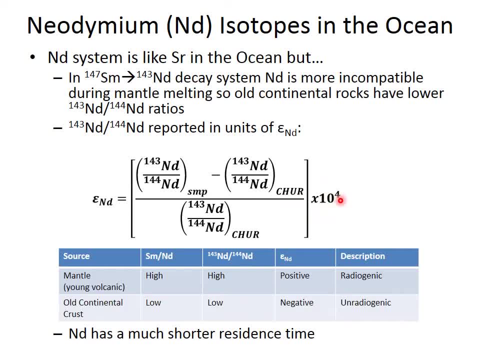 And this is basically changes by parts per 10,000.. So small variations, okay, And they're driven by. Well, you can go back to the beginning of the lecture and find out what causes those changes, But the important thing is neodymium has a much shorter residence time than strontium. 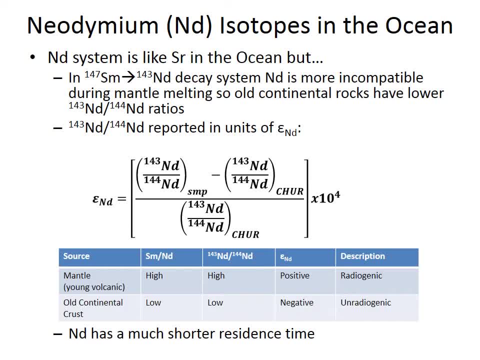 Okay, So the residence time of neodymium in the ocean is of the order of maybe hundreds of years, So we do see variations in the isotopic composition in the ocean. Okay, so this is basically some measurements of the composition of the sources. 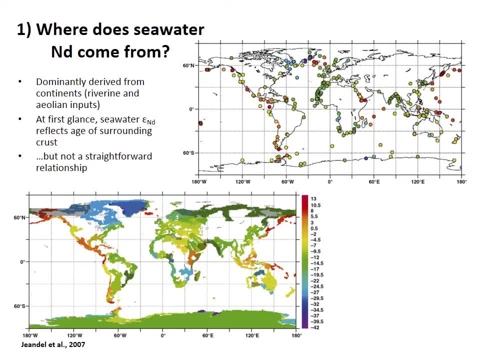 So the neodymium in the ocean ultimately comes from weathering from the land, very similar to strontium, But different parts of the land have got different neodymium isotope compositions. Okay, so old bits of the land will have had less. 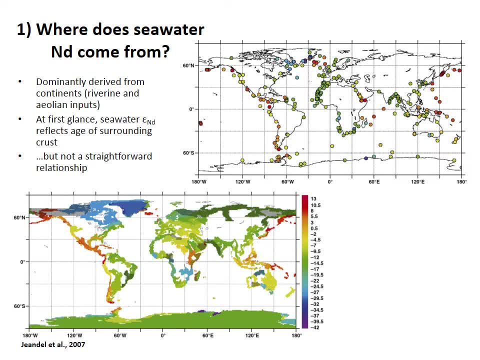 will have Old bits of the land, will have less samarium than neodymium, because the samarium is basically hidden away in the mantle, So they will have. So places like Greenland and Canada, Canada, Canada, Canada, Canada. 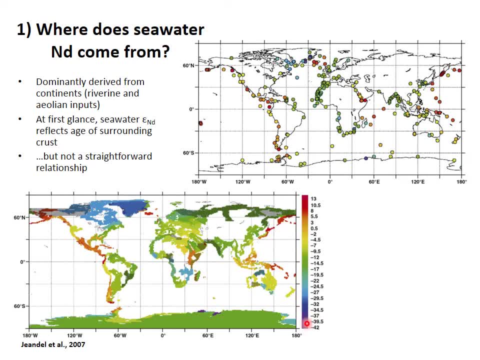 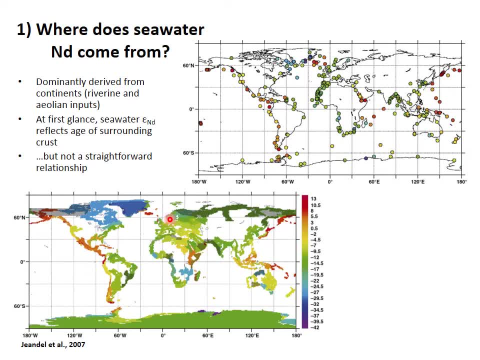 Whereas younger rocks. okay, they have had chance. but before they were formed, the samarium in the mantle could grow into neodymium and then, when they were formed, that neodymium would have then a slightly higher 143-144 ratio. 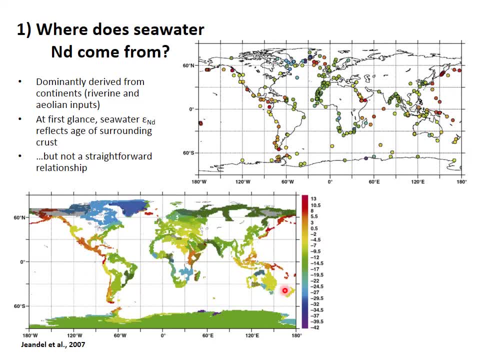 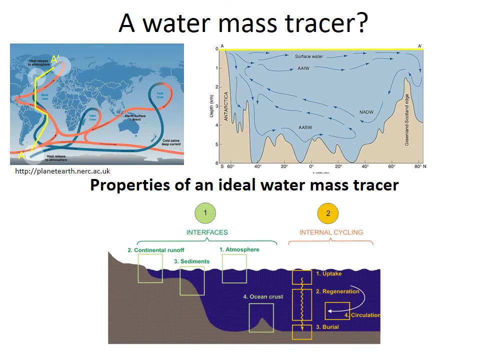 But basically, you know, old rocks- low numbers, young rocks like high numbers. Okay, volcanic rocks- low numbers. So we're going to see how neodymium isotopes can be used to trace water masses as they move throughout the ocean. 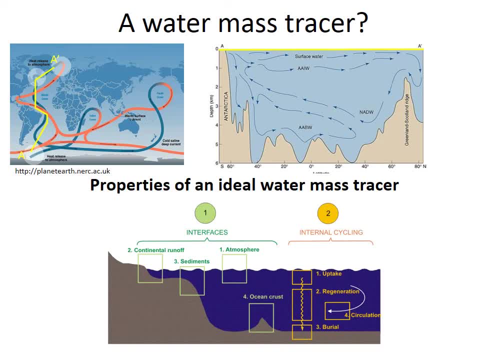 So hopefully you will be familiar with kind of the top two diagrams. This is kind of like the schematic ocean conveyor of how kind of deep currents move around the Earth, So in, for instance, here This is across basically this yellow line. is this yellow line up here? 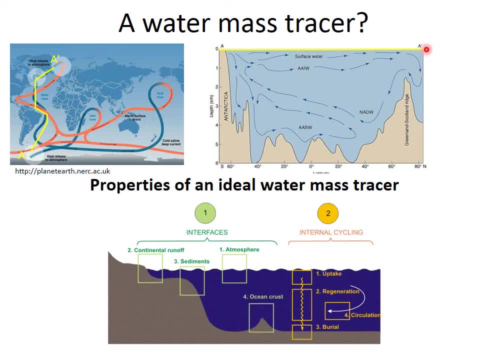 So we're looking at a section through the ocean. So in the North Atlantic here deep water sinks okay, then flows up and up wells in the Southern Ocean where it then forms something called Antarctic Intermediate Water and Antarctic Bottom Water, which fill kind of the oceans flowing back to the north. 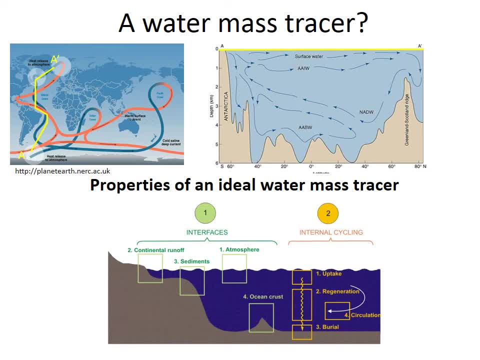 So if we want to figure out where those water masses are, now that's very easy. We can just measure the temperature and salinity of the water and that tells us kind of pretty much where that water came from. and we can kind of kind of 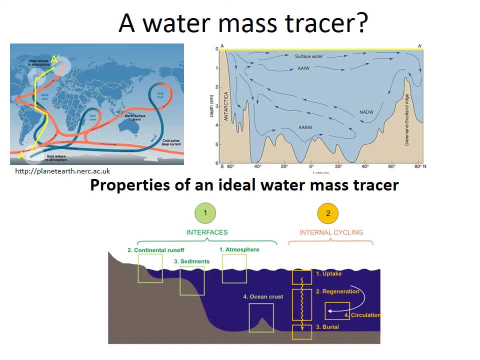 label the water masses. but in the past: okay, it's very, very hard to measure the temperature and salinity of seawater. from the past: okay, because we don't have the water. Okay, we can measure proxies for it. 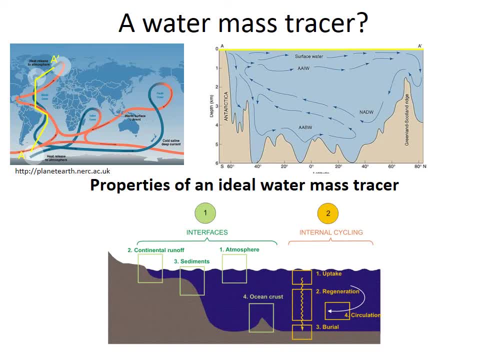 but one of the things we can do is we can see, if we could. there is some other basically geochemical label that's basically attached to the water masses, okay, and then gets preserved in sediments, Okay. so this, this bottom thing, is basically describing what would make a good 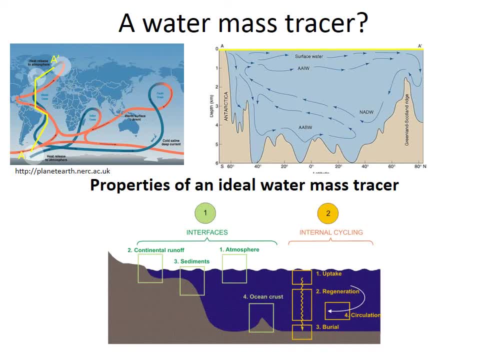 what would make a good proxy for that? So we want something that basically doesn't get changed, so it won't change the composition of the water mass tracer when it's in the water mass. It will only be affected when that water mass touches basically the edges of the ocean. 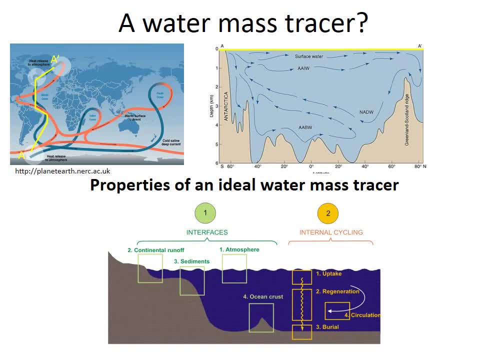 So its composition is set at the boundaries but not changed in the interior and also it doesn't- it's not- affected by biogeochemical cycles. okay, because that would change the composition of the tracer as it was moving along in the same water mass and that would mean we couldn't use it to trace the water mass. 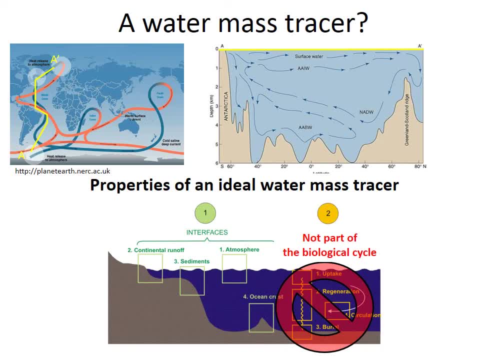 So neodymium is quite good for this, because it's not part of the biological cycle at all. okay, and it is only really set by exchange with the boundaries. Okay, so where the water meets the edge of the ocean, either at the surface, the addition of dust or the interaction with sediments, 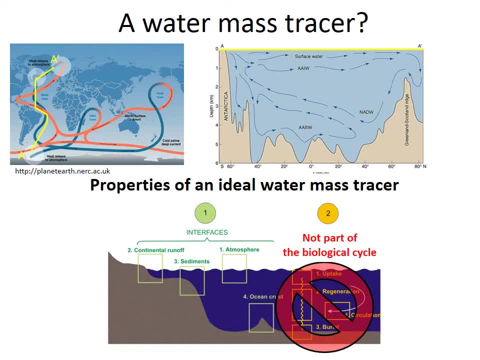 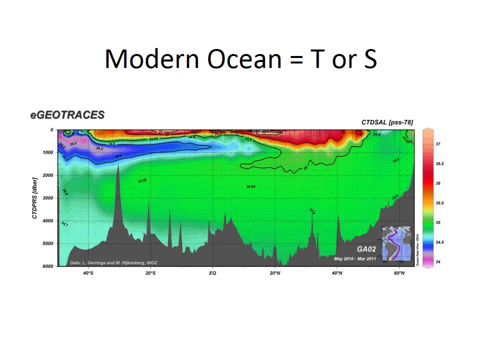 that can change its neodymium isotope composition, but when it's in the interior of the ocean it can't really change much at all. okay, so this is, this is a. this is that same section. so we can see here: this is the. i think this is the salinity, so we can see here the salinity. quite nicely, this. 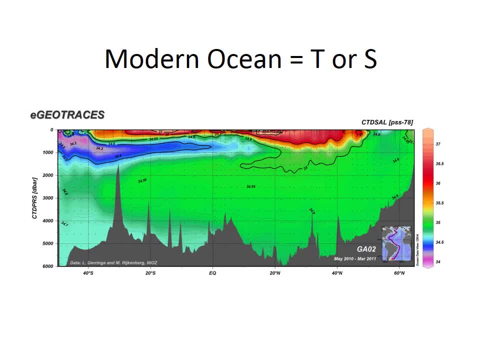 green tongue picks out. well, for you, green tongue. uh, the green tongue picks out the um north atlantic deep water forming in the high north atlantic, and then the blue water masses. the ones with lower salinities are those antarctic intermediate and antarctic bottom water, so we can use salinity. 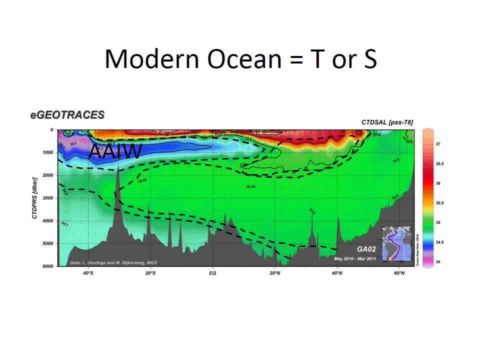 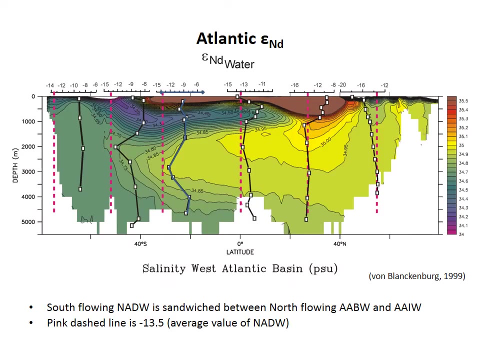 to pick out the water masses in the modern. okay, and those are those water masses. that was fancy and there are more that you. there are lots and lots of different kinds of water, but if we now look at measurements of neodymium isotopes, so the background color on this is still 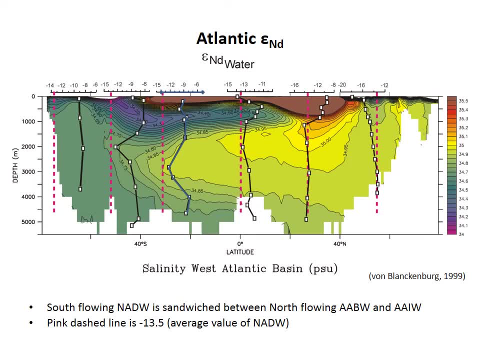 the modern ocean salinity and the. the profiles are the uh, our measurements of neodymium isotopes. so it's all hardest to measure neodymium. so there are many, many fewer measurements. but we can see here so that the, the, the pink line in each of. 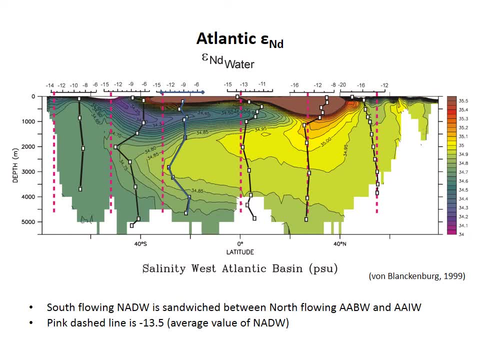 these graphs is kind of. i think it's 13 minus 13.5 epsilon value. so you can see in the north atlantic we've got uh, something that's close to minus 13. then as we move down through the uh, the blue water basically maintains that same value. okay, but the uh, uh and the antarctic intermediate. 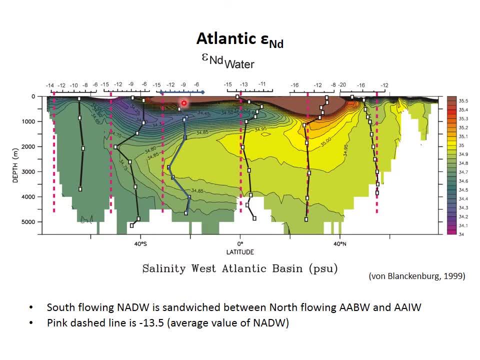 water coming in here that has got a higher neodymium isotope ratio. so that means a less radiogenic okay source which is similar to the rocks around the southern ocean, similar to the, the deep water down here. so that's got, um, uh, a more positive, less radiogenic neodymium isotope. 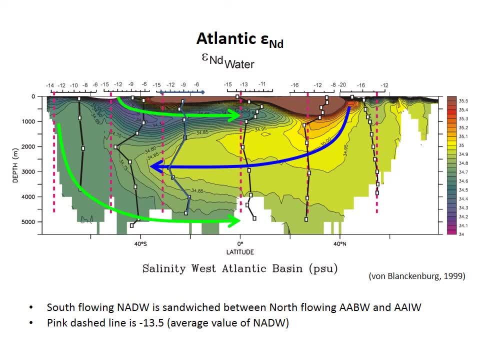 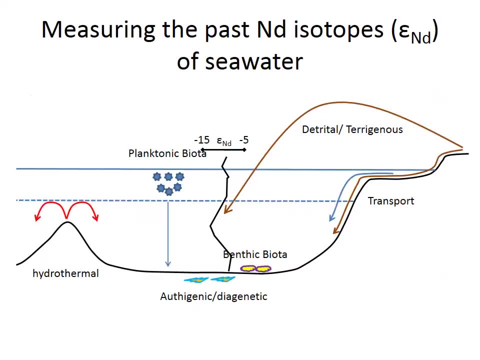 composition here, so we can use, then, the neodymium isotopes, in this case, to identify the water masses. if we're going to use this to go into the past, we can't measure the neodymium isotope composition of the water, because the water isn't there anymore. okay, so what we have to use is something. 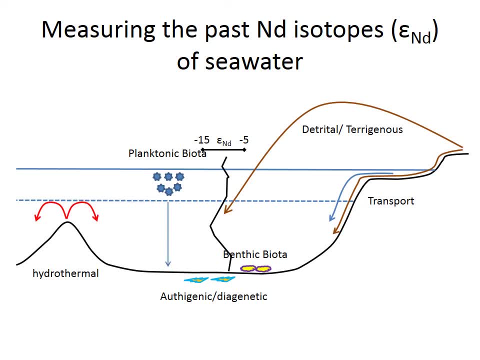 that has basically captured the neodymium neodymium from the water and preserved it in sediment. okay, but we don't want kind of the whole water to be in the water. so we can use the neodymium isotopes to identify the water masses column composition. we just want to know what it is at each level in the water. okay, so we want to know. 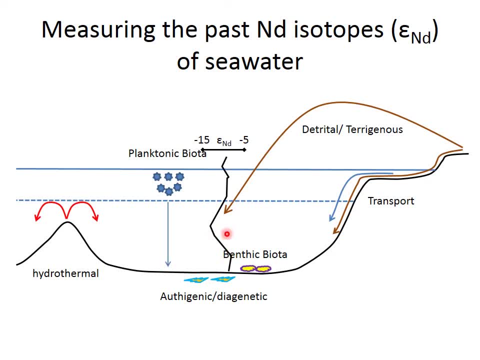 what the neodymium concentration was here, was here, was here through back through time. okay, so we want something that's grabbed neodymium from, say, this level in the ocean and preserved in sediments, okay, so if we just wanted to know the surface, we could, you know. 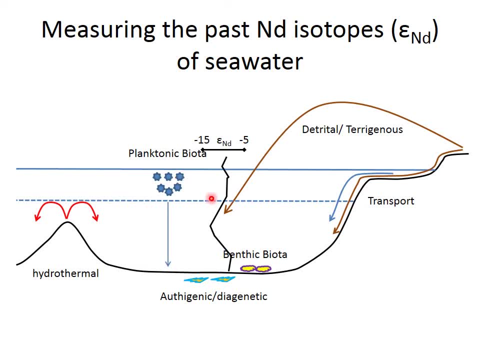 measure some planktonic foraminifera, okay, but if we want to know throughout the whole water column, what we have to do is get rid of that arrow and basically have it go somewhere in the ocean where the sea floor basically rises up through the water. 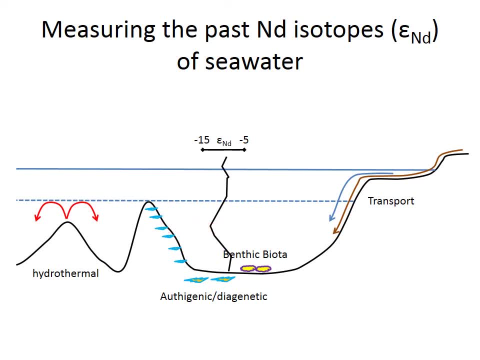 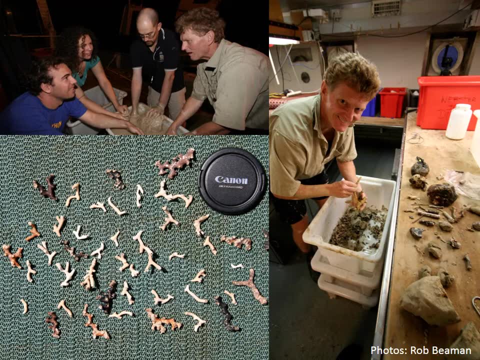 you, you, you, you. so this is uh, this is our head of department, uh, who was on a research cruise with me ages ago now, and these are corals and those corals were living on the sea floor and you can see that some of the corals are white, okay, and that is the color that the coral should be, okay, and then some of them are. 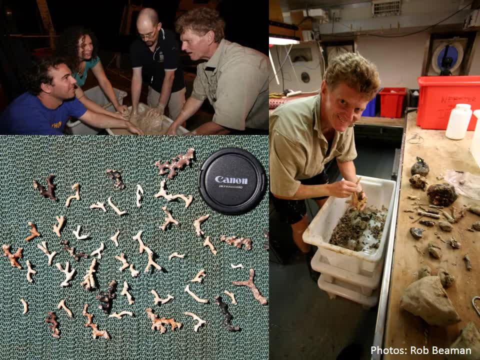 quite dark colors. okay, so there's some blacks and some reds, and what those are is those are iron, manganese coatings that are formed on those corals once they've died, and those coatings are basically scavenging rare earth elements from seawater. so if we basically collected samples like this from a depth profile throughout the ocean? 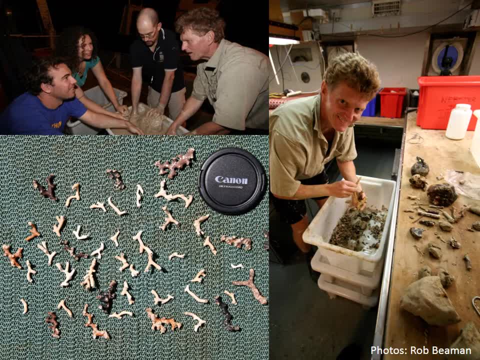 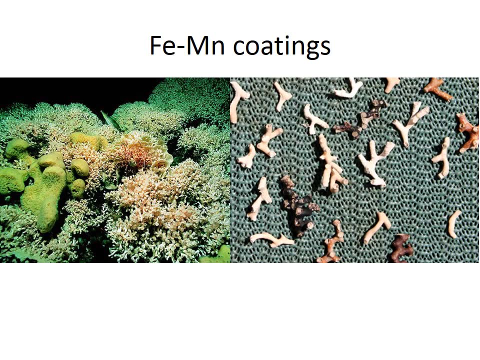 at each level, we'd be able to record the neodymium isotope concentration and composition from from the from the seawater. okay, so this- i mean this is this- is on the: on the left, there, that's what they look like when they're living, and on the right, here you can see that they've got these, these dark coatings on them. 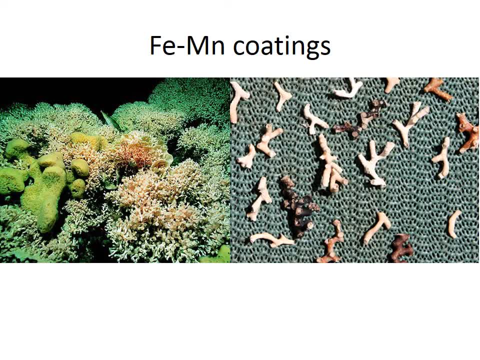 which has enabled us to basically extract neodymium from the seawater. now you don't have to get corals, they can be anything that's precipitated from seawater. so some uh on, if you can even just sediment grains, develop these iron manganese coatings. so if you can isolate the iron manganese coating from the 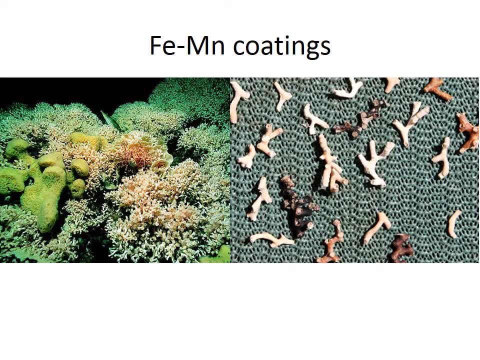 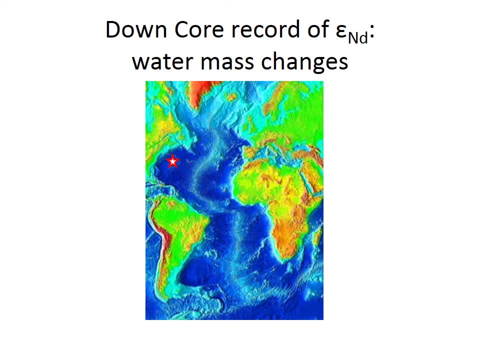 rest of the sediment, then you can use that to reconstruct the isotopic composition of seawater. so just some examples of that. so this is from the north atlantic um. so before we go into the north atlantic um, we've got all the islands and the seawater. there's a lot of sediment in there. 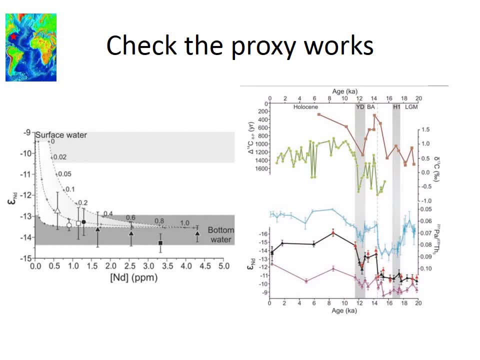 but before we kind of like move on and and use these records down core, we basically need to make sure that our proxy works. so what we've got on the left here is basically an experiment to test whether we can extract the the right isotope ratio from sediment. so these are, uh, planktic. 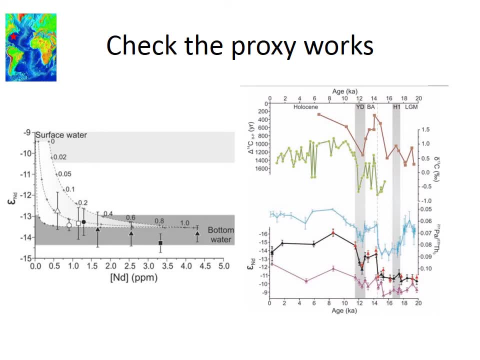 foraminifera that lived in the surface ocean, okay, and they've sunk down to the bottom of the ocean. they've died. and once they're sitting on the sea floor, they've got these iron coatings on them, okay, So what's what's happening here? and those coatings have got are basically enriched in neodymium. 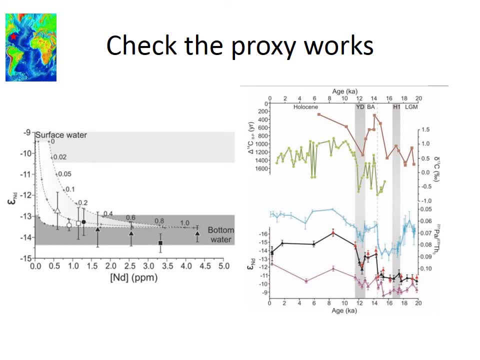 The coatings, basically, are good at grabbing rare earth elements from seawater, whereas the the, the 4M calcite, has got a much lower concentration of neodymium. So what they've done is they've they've measured the composition of the water at the, at the core site, at the bottom and at the surface. 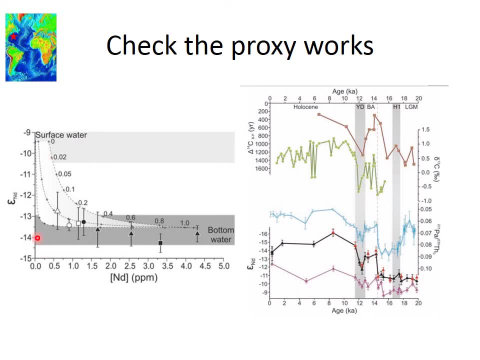 And you can see that they're different ratios here: okay, minus 14 and minus 10.. And then they've taken the 4Ms, okay, and they- this was just measured- the 4M, okay. and then they've cleaned it a bit to try and remove that iron coating and they've measured what's left. okay. 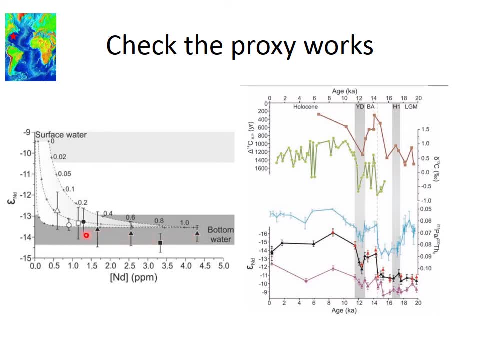 And then, as they do that, they carry on cleaning it. it gets less and less neodymium concentration as you keep on removing that coating. okay, until you remove the coating completely, And then you start to change The isotope composition as you start to have a significant component of the original calcite. 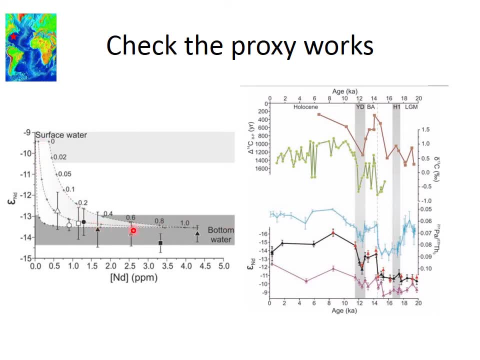 So this basically shows them how much they need to clean their 4Ms to make sure that they're clean and don't have any stuff that's maybe clays or something that might have a different isotope composition but has not changed the isotope composition beyond what like outside of the the range that represents the seawater value. 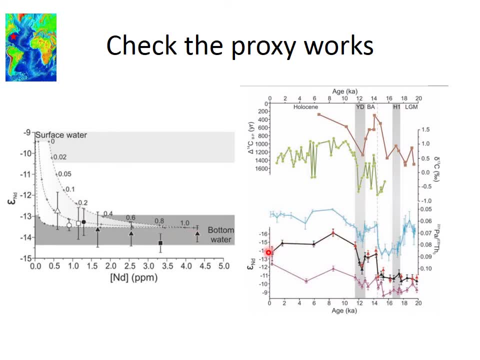 So that's what they've done: Uh, downcourts. So this is the sediment core as well. so if you just look at, so this is a a bunch of measurements in the sediment core. it doesn't really matter what's going on at the top up here, but down here this is age, and just look at the um, the black curve here. so these are neodymium isotope compositions of uh, two different things that have, um, uh, uh, basically been sat on the seafloor and grabbing neodymium. 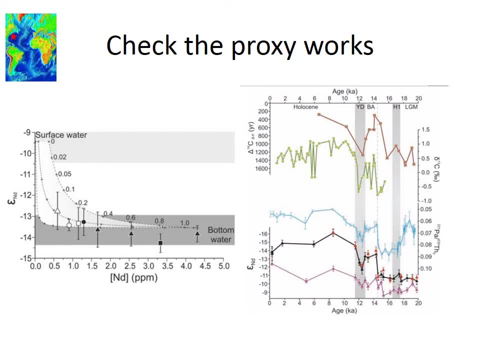 So one is these 4Ms that fell down to the bottom and they've got these coatings on, And the other is fish teeth. So it turns out that fish teeth- or in fact any kind of teeth, uh, when they, when they sink to the ocean floor, they basically start with no rare earths in them, no neodymium, and then they basically start to absorb rare earth elements really, really quickly. 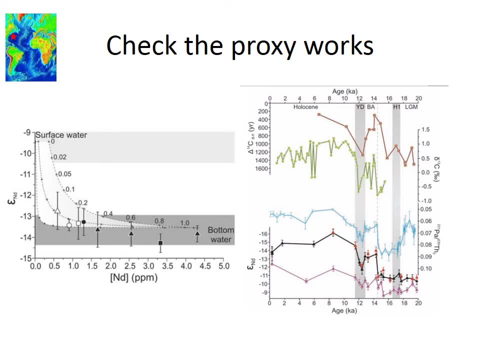 Um, that's quite a good question, um, but I don't think anybody knows the answer. Um, it's, I think it's a, it's a property of the, the hydroxyapatite structure, Uh, and that subtly changes. so it's basically got- uh, it's got, rather than just being apatite. it's got small amounts of calcite in it as well. 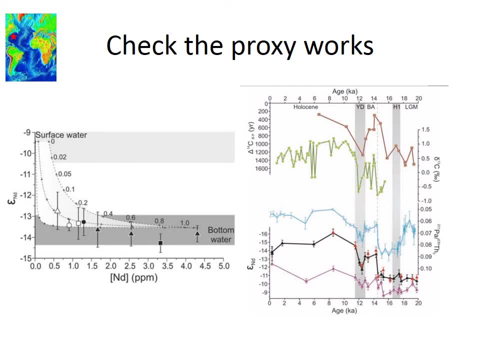 And that basically it creates quite a porous kind of network of of mineral and because it's got lots of edges of mineral, that's got basically a high um affinity for stuff. Um, uh, so it happens with bones as well. 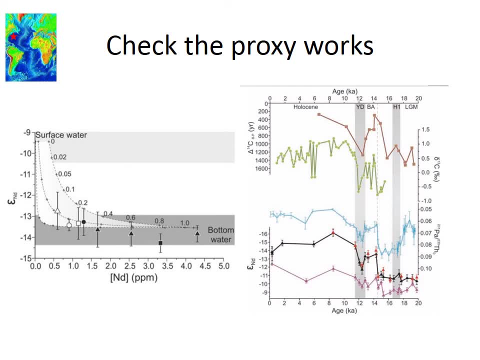 So if you, if you go and measure, say, bones from some archaeological sites, you'll find they've got huge compounds, Um. so you can see that there's huge concentrations of trace metals, Um, and that's just because they've absorbed them from the environment around them. 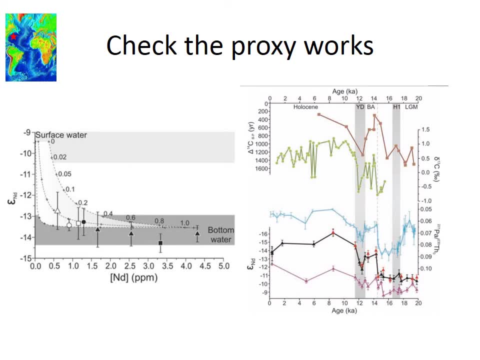 Um, So would like calcite always have more or less. So pure calcite would have less. So it's not. it's not that it's got some calcite in it. It's basically that it's got lots of holes in it where the calcite is. 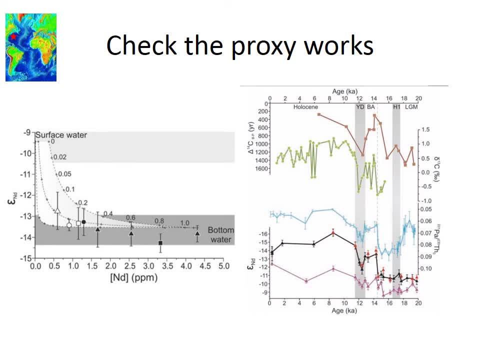 Um, so it's basically it's like a it's got mineral. it's mineralogically it's a bit like a sponge. but what basically? they've measured: the black triangles and the red triangles are the same sample of sediment, and they've measured the fish teeth and they've measured. 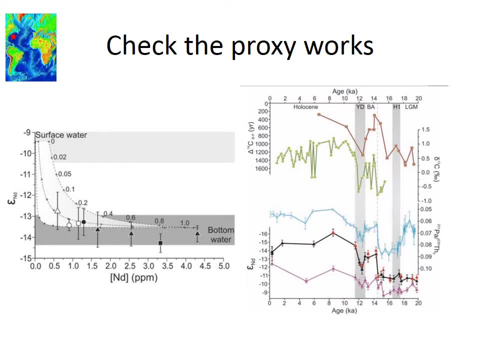 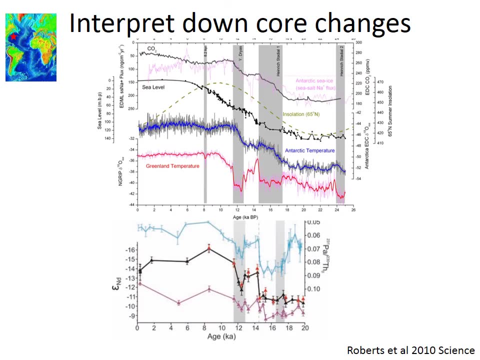 the forams and they've got the same number. They've measured two different things, got the same number. That gives you some confidence that you're getting the right number. So just to put these kind of data in context. so the top gives some kind of background to what's going on climatically. 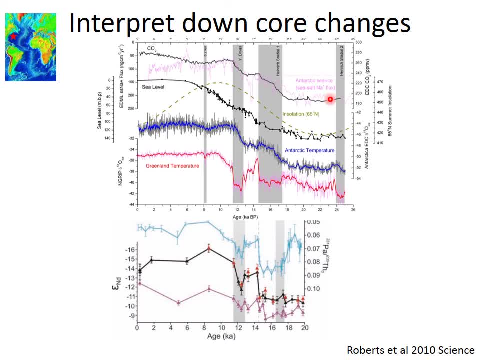 in this kind of time frame. So we've got at the top here. the black is the carbon dioxide concentration in the atmosphere. so this is increasing across the deglaciation Sea level, going up quite dramatically across the deglaciation Changes in Antarctic temperature. 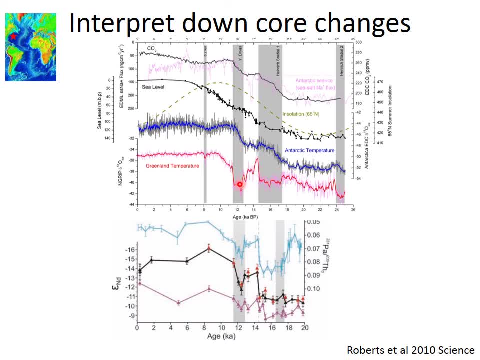 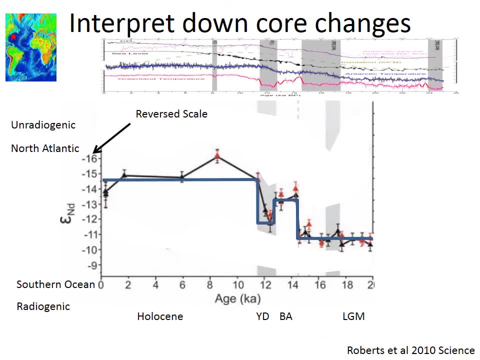 that are quite different to the changes in the temperature in Greenland. And then here down here we've basically got, I think, on the next slide, okay. so if we then zoom into this bottom slide here we've got the neodymium isotope composition. okay, so this. 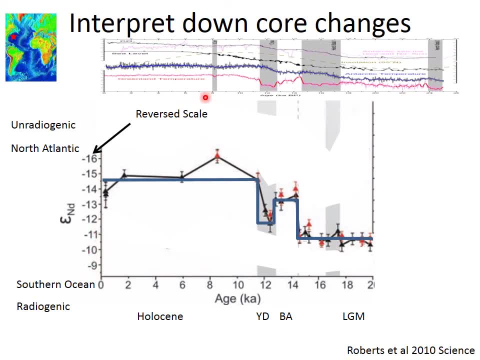 is the scale. Paleoceanographers really love to screw with your mind and flipping scales around all over the shop. So we've got unradiogenic. so for neodymium that means the old rock source up and the young rock source down. so more radiogenic down here. 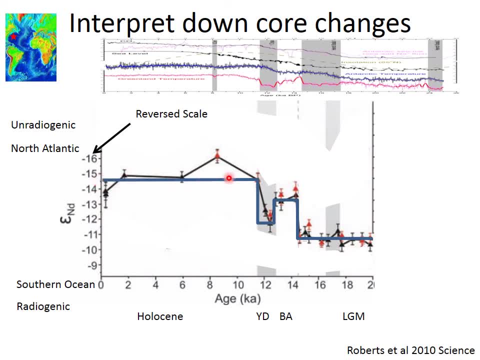 So in the Holocene we've got arm the fairly- you know, uniform ish signal that basically looks like it's getting its neodymium from the North Atlantic, from all those old rocks around Greenland. Okay, but then back in the Glacial times. 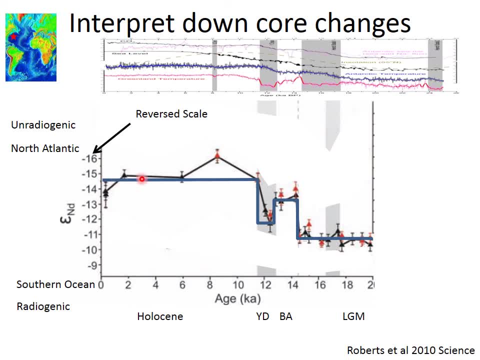 you can see, the neodymium isotope composition is much lower, much higher. on this it's flipped axis, so it looks like it's getting it's neodymium from somewhere else that's got little more activity to it. So this is just more households that are getting neodymium from Greenland. 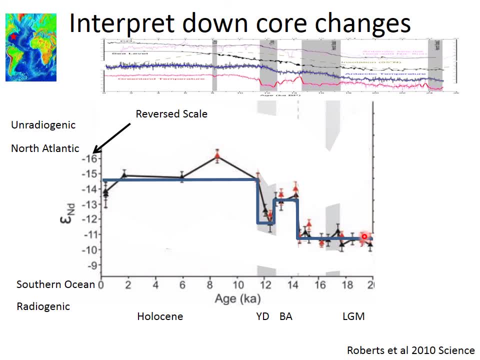 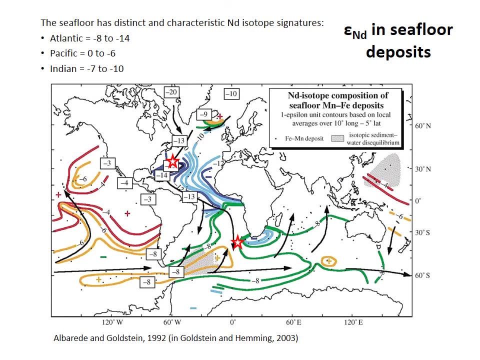 got much more volcanic rocks, okay, and then you have these little ups and downs during the deglaciation, okay. so if we look at just a map of sediment isotopic composition now, we can see that this kind of maps out, uh, so we've got these, uh, these very low, very unradiogenic. 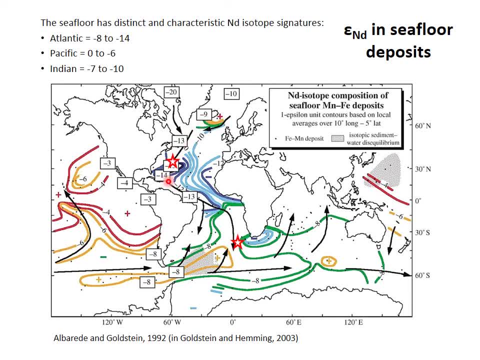 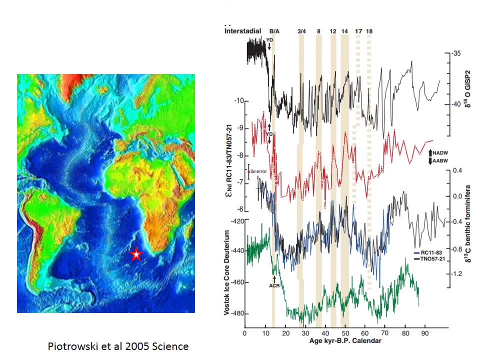 neodymium isotopes up here in the north atlantic, and you see that the pattern kind of follows the flow of deep water. okay, so for now we've got another sediment core down here in the south atlantic, um, and this red curve is the one you want to be focusing in on. so once again, we've 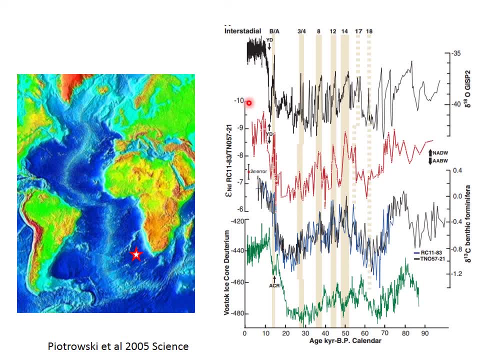 got here the neodymium isotopes. once again the scale is flipped, because you know we like to do that to you and we've got more negative, more north atlantic type compositions up here in the holocene, more kind of southern ocean, more kind of- uh, less sorry, more radiogenic neodymium isotopes down here in. 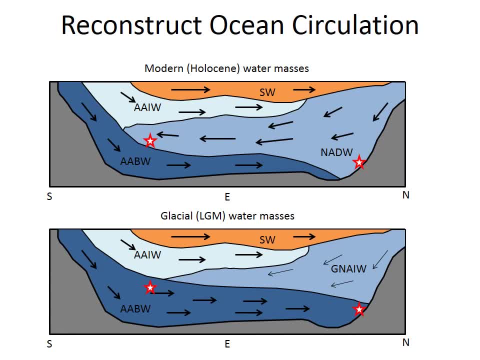 the glacial period. so we can now start to use these to kind of reconstruct how we think the ocean circulation was in the past. so the top figure is here: this is a holocene configuration where we've got north atlantic deep water flavored neodymium in our northern core site. 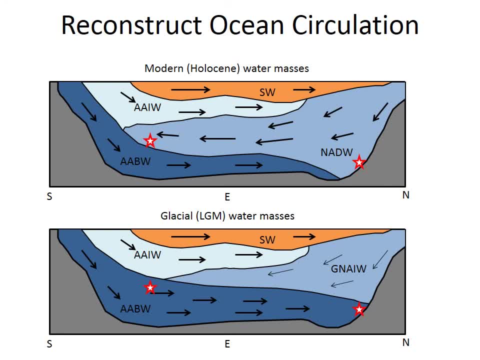 and kind of similarly north atlantic deep water flavored uh water in the um, in the southern ocean. well, in the where we've got our core site, okay. so the core is basically floating up in this section because it's sitting on a uh, it's sitting on the continental margin, so it's higher up in the ocean. 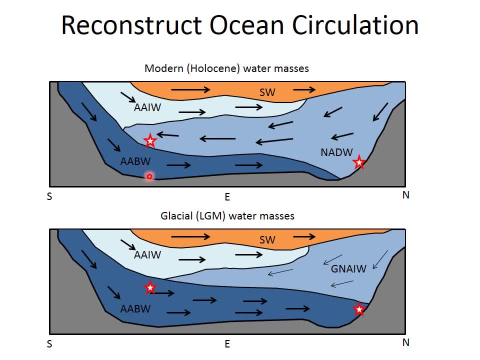 so it's sampling this shallower water than being at the bottom um, but in the last glacial maximum both of the core sites have a neodymium isotopic composition that represents more of the southern source, more of the the radiogenic uh kind of neodymium isotopes that are found in the. 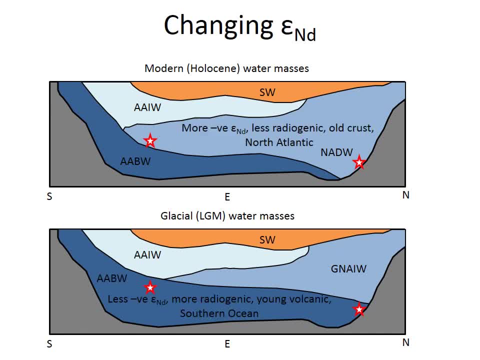 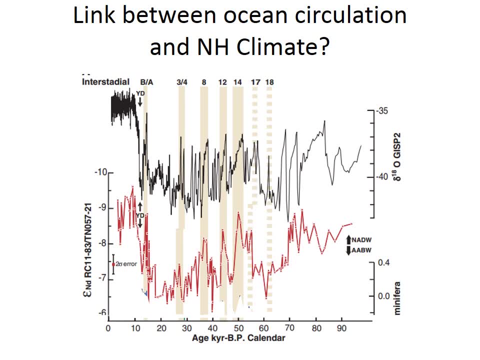 from uh rocks around the southern ocean. okay, so that that kind of summarizes what i've just said. um, and this is kind of important because we can now have a- we basically now have a record of uh, how oceans the ocean was circulating. okay, this basically the, the, the relative strengths of 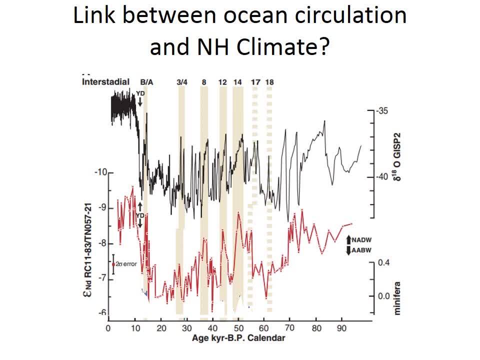 deep water formation in the northern hemisphere versus deep water formation in the southern hemisphere. so in the holocene we've got more deep water being forced formed in the northern hemisphere, coming down into as far as the southern ocean, whereas in the glacial maximum down here we've got that north atlantic. 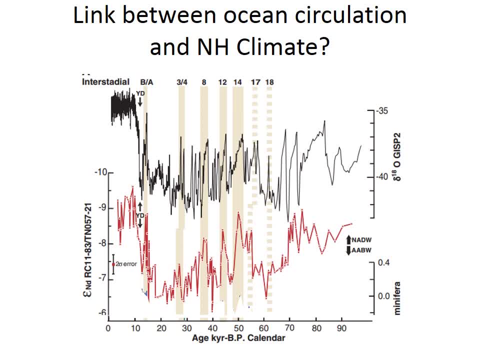 deep water signal is much, much less strong and we've got water filling the whole atlantic from the south. okay, and you can see the impact of that on the temperature of greenland. okay, so you can see that these changes in how the ocean is circulating are really tightly. 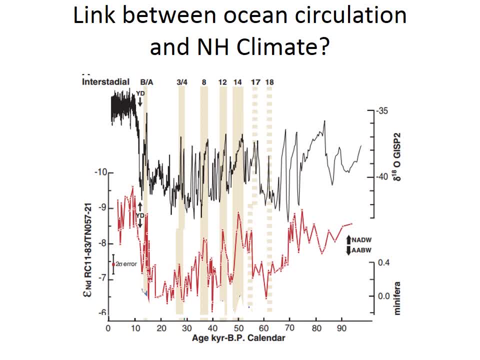 coupled with how, uh, the earth's climate is. so this is north, basically northern hemisphere temperature. so these dramatic swings that we get in northern hemisphere temperature are closely linked to how, how, the ocean is circulating. now, with these data, we we're as yet unable to say which is the car, and 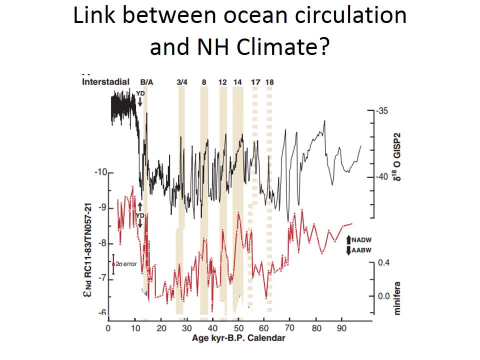 which is the horse? so which is which is driving what? so is it the temperature changes that are changing ocean circulation, or is it ocean circulation changes that are driving the ocean? so we're driving temperature change. okay, it's likely not as simple as that either, or they're probably. 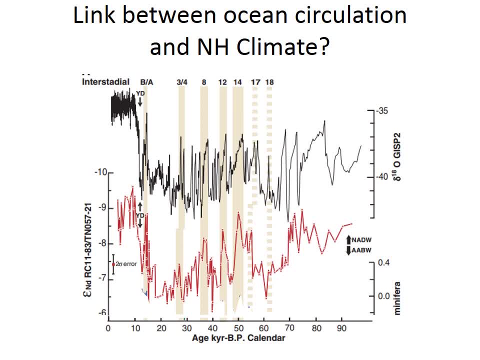 tightly coupled, but just to point out that we can actually now use our radiogenic isotope knowledge to tell us something actually quite useful and interesting about paleo climate. okay, so those of you that sat for all of jeff's lectures and wondering where the hell it's going, why we're